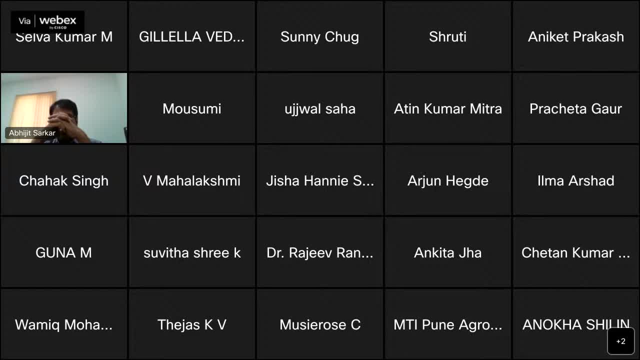 Dr Sarkar also takes very active part in capacity building. in recognition of his outstanding scientific contribution in the field of atmospheric sciences, He was awarded certificate of merit by the ministry of earth sciences government of India in the year 2016.. I now welcome Dr Abhijit Sarkar to continue his lecture. 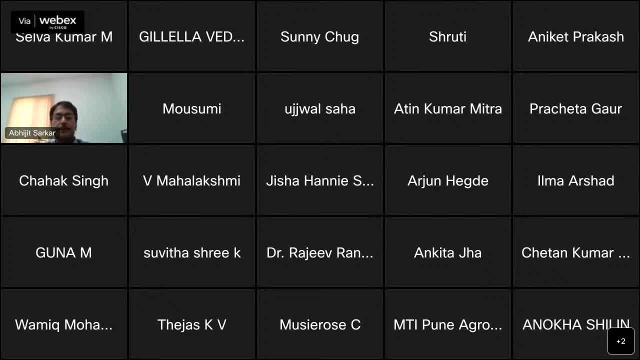 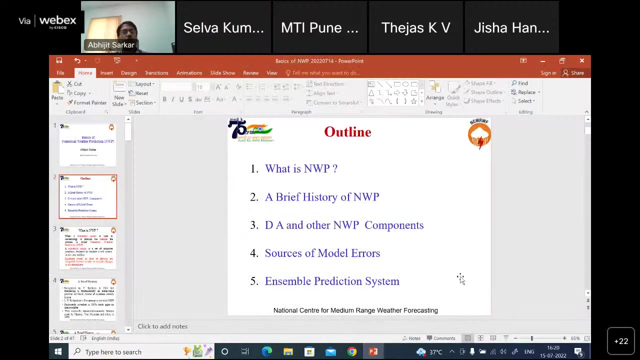 Thank you for your very nice introduction. So now I am trying to share my PPT. Okay, Is my PPT visible? Yes, sir, it's visible. Kindly do in presentation mode, sir. Yeah, I am making full screen. Yeah, now it is okay. 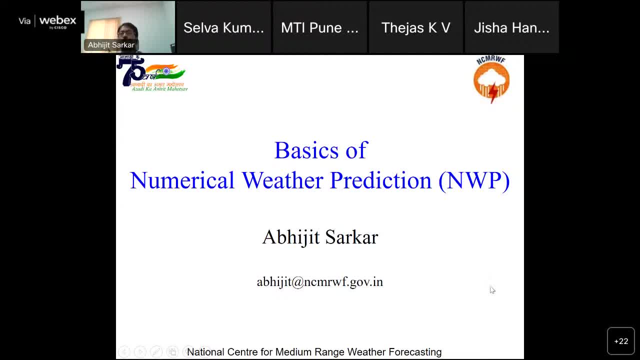 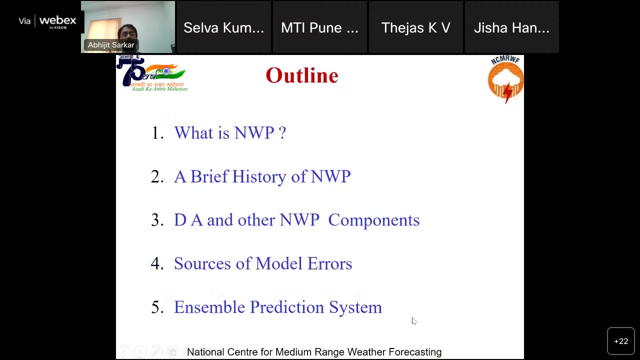 Yes, sir. Okay, thank you. Hello, Good afternoon everybody. Today's of today's topic talk is basics of numerical weather prediction. so in today's talk i will cover this. what is nwp? a brief history of nwp, then data assimilation and other. 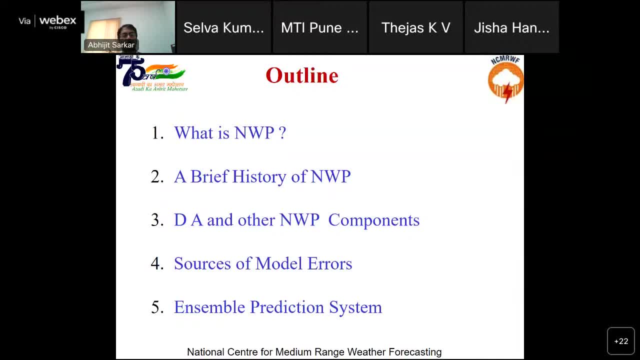 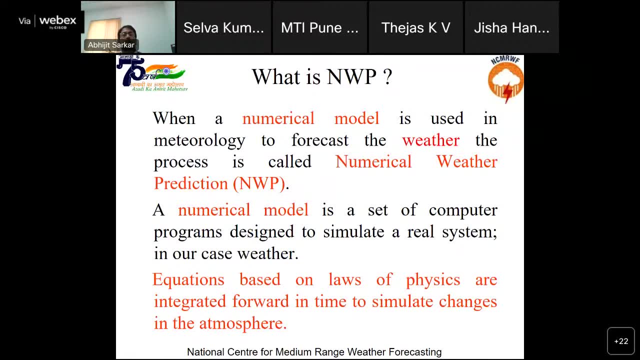 nwp components and sources of model errors and ensemble prediction system. when a numerical model is used in meteorology to forecast the weather, the process is called numerical weather prediction. so a numerical model is a set of computer programs and this set of computer programs is are is designed to simulate atmosphere or weather. 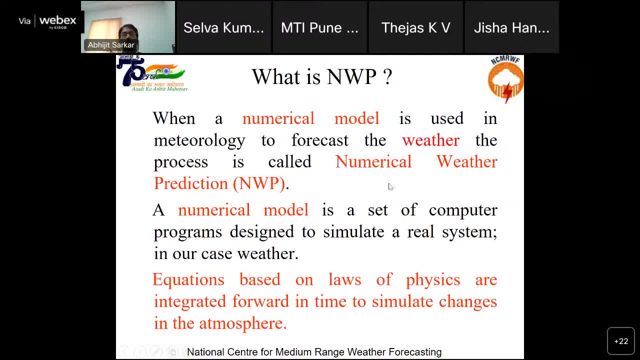 so a numerical model is a set of computer programs, and this set of computer programs. now, how do we write this set of computer programs? first, we take the equations based on laws of physics that govern the atmospheric motion. those equations we write in the form of differential equations. 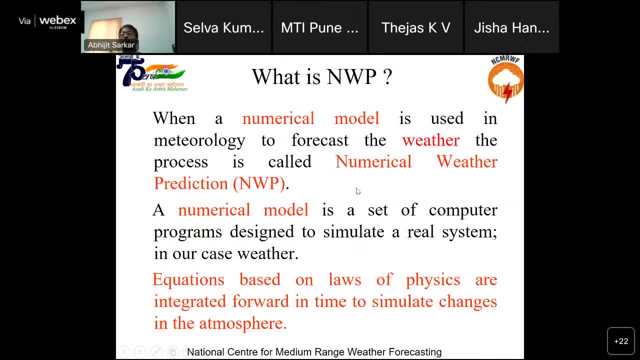 and then we solve these differential equations. so that means we integrate forward in time to simulate the changes in the atmosphere. and this solution method we write in the form of program, so when this program is run within the computer so we can tell that artificial weather is evolving within the computing system. 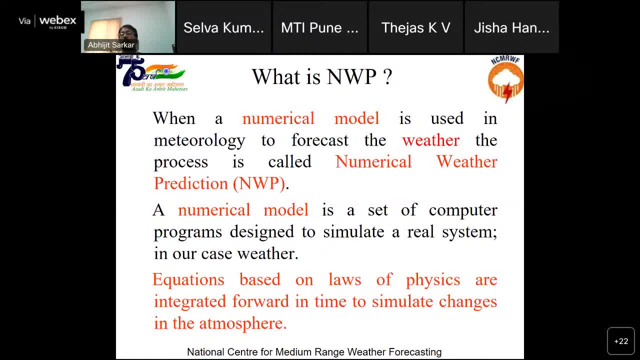 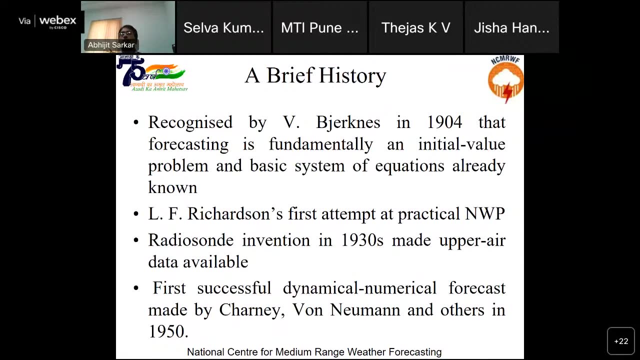 so, starting from an initial condition, we will integrate those equations to get the future state of atmosphere. so before going directly to this numerical weather prediction or nwp system. so let us first discuss about a brief history of nwp. it started with v vartnes in 1904 and he only conceived this idea that forecasting is. 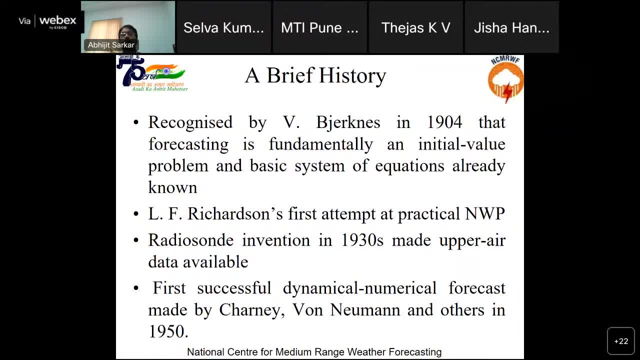 fundamentally an initial value problem and he only conceived this idea that forecasting is fundamentally an initial value problem and basic system, basic system of equations already known. so basic systems of equations means this, means that's equations for the conservation principles. in 1922, first la richardson son tried, tried to implement that idea of 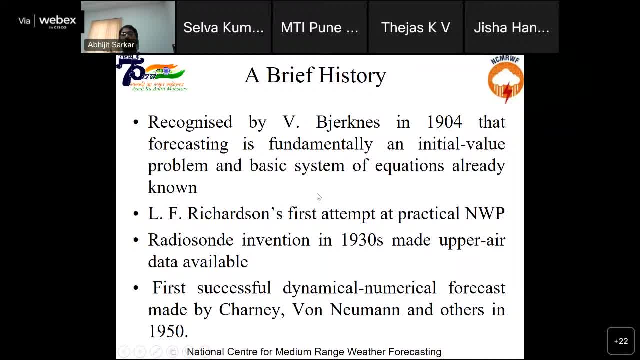 vartnes and he tried to calculate the pressure change in six district of unit area for hours but somehow his calculation was wrong and it is well known why his calculation was wrong. but what he anticipated? he anticipated that maybe more than 60 000 human computers if we put 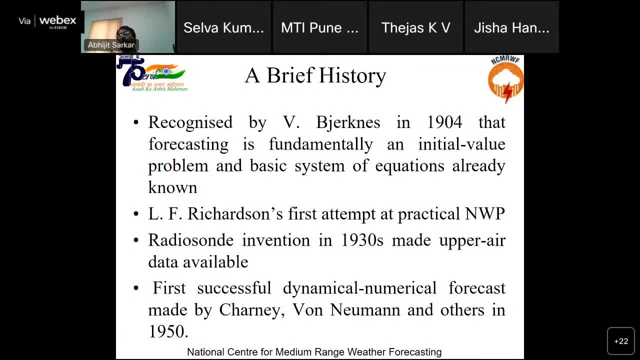 for the whole globe. so then we will be able to compute correctly the weather systems and in time, because richardson took a long time, more than six week, to calculate six hours weather change and in six hour he found out that the weather has changed about this pressure. surface pressure has changed about 100, 145 hpa, which is unrealistic. 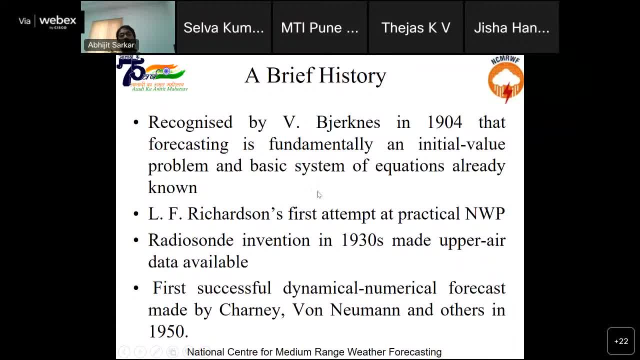 so today we don't have so many human computers around the globe, but we have hpc's high performance computing systems, which are used for weather forecasting, global weather forecasting- and after that, in 1930s, radio sunday was invented. and with the invention of radio sunday, 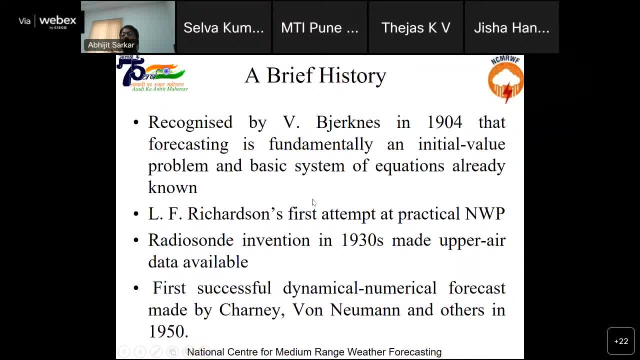 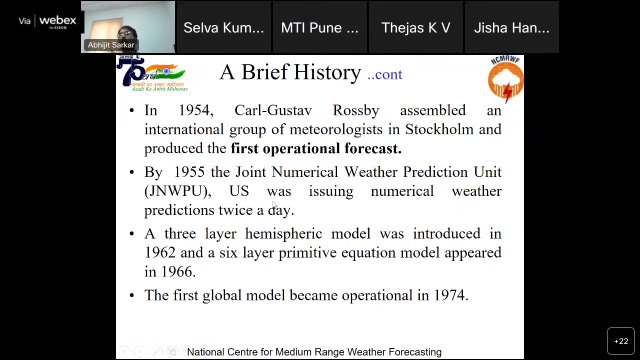 the information from different levels of the atmosphere. vertical levels of the atmosphere. they started coming and before 1930s only the observations at the surface level are available and first successful dynamical numerical forecast was made by charney von neumann and other researchers, inhil nella bain. this observation was studied on paper whenever continually. 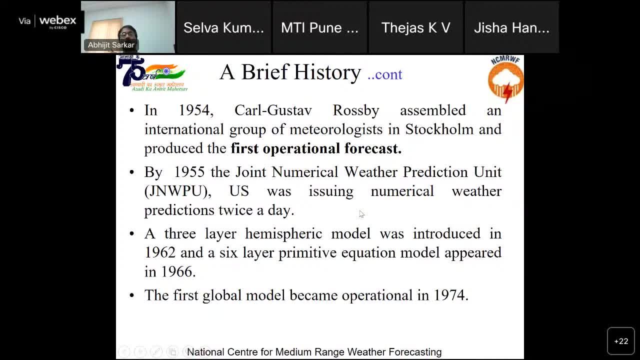 the oxygen of the air was enough to befaol, gripped not just by sensing but by observing, and sacrificed by the眼界 scientists including john brilliant, obama trajan and karen bodigal Starler. essential找枠. weather prediction twice a day. A three-layer hemispheric model was introduced in 1962. 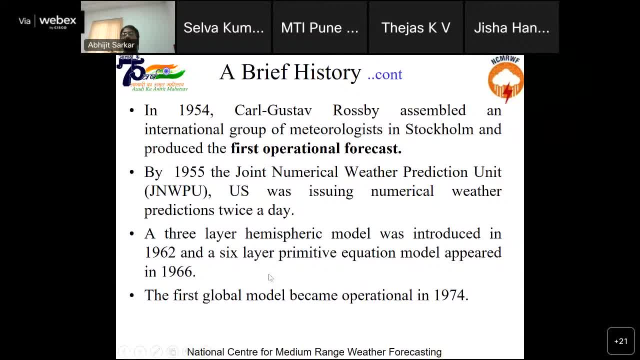 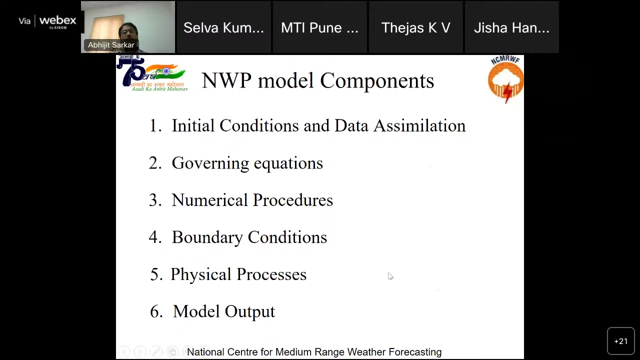 and a six-layer primitive equation model appeared in 1966 and the first global operational forecast was done in 1974.. NCMRW started giving global operational forecast in 1990 around. So there are several components of NWP. First is initial conditions and data assimilation. 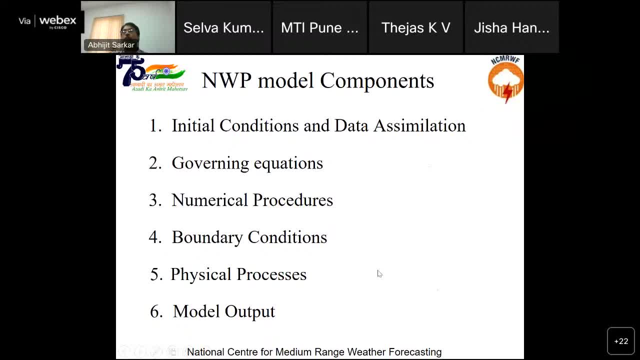 then the formulation of governing equations, then the formulation of the NWP and then the formulation of the NWP. So there are several components of NWP. First is initial conditions and data assimilation, then method of solving these governing equations using numerical methods. 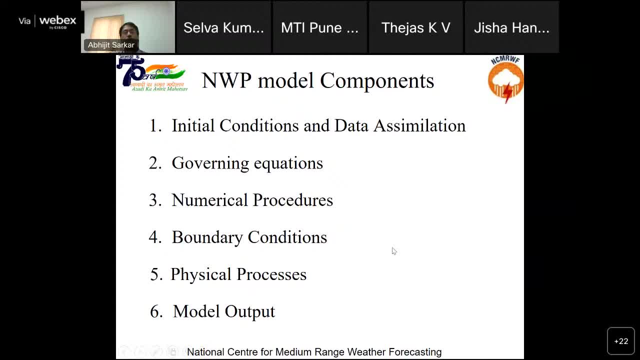 then implementation of boundary conditions, parameterization of physical processes and finally, the model of. I will briefly discuss about all these points. So first let us start with initial condition and data assimilation. So, as I have already told that NWP is an initial, 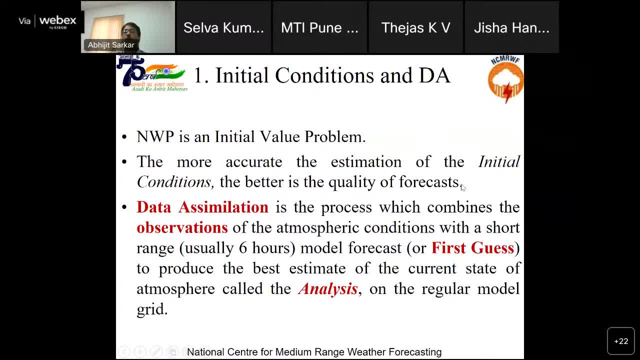 value. So let us start with initial condition and data assimilation. So as I have already told that NWP is an initial value. After這一азывание, if you solve the problem with linear acceleration, the final outcome- 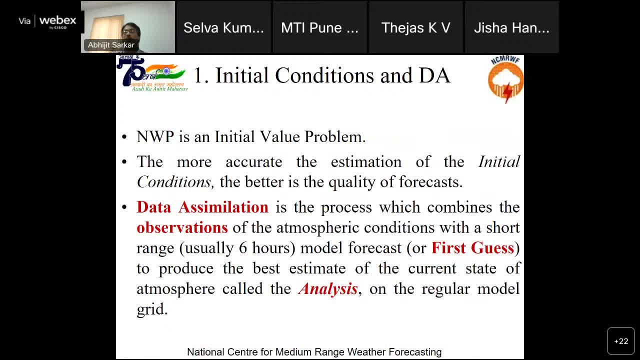 depends on the initial condition. then if the initial condition is very accurate, then the quality of forecast also really good, particularly weather forecast. If we go to the longer range, so more and more longer range will go. Voluntary conditions also will become more and more important in this way because the global 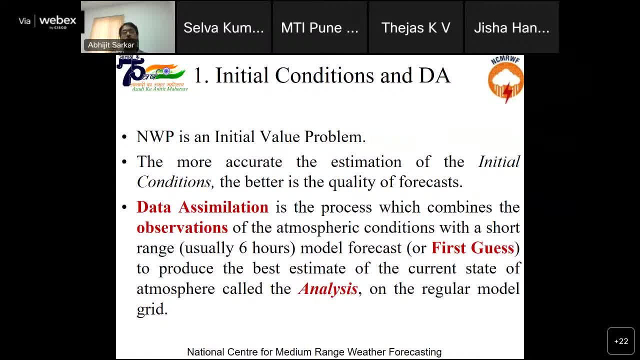 more important and initial condition will not be that much important. but we are talking here about weather prediction, not climate prediction, so it is an initial value problem. so we have to take care of preparing the initial condition and the method of preparing initial condition by combining two information. 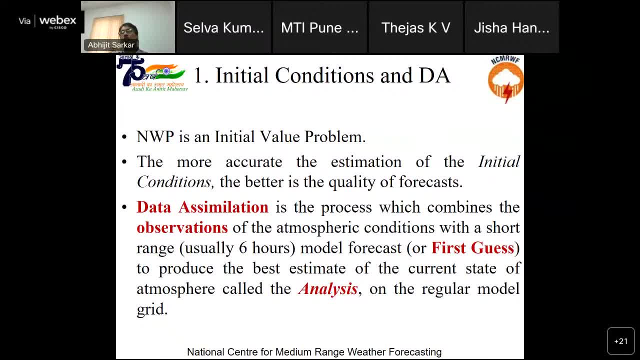 one comes from the short model forecast or first case, and another comes from the observation. it's called data assimilation, and the prepared initial condition or the best estimated state of the atmosphere is called analysis. so data assimilation is the process which combines observation of the atmospheric condition. 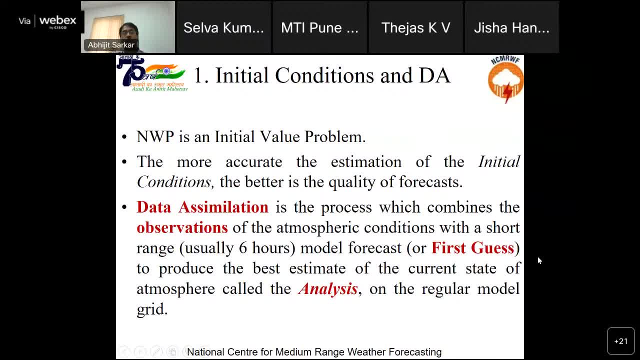 with a short range model forecast or first case, and the data assimilation to produce the best estimate of the current state of the atmosphere, called the analysis on the regular model grid. so we have two information: one information comes from the observation and another information comes from the short model forecast or first case, and both are 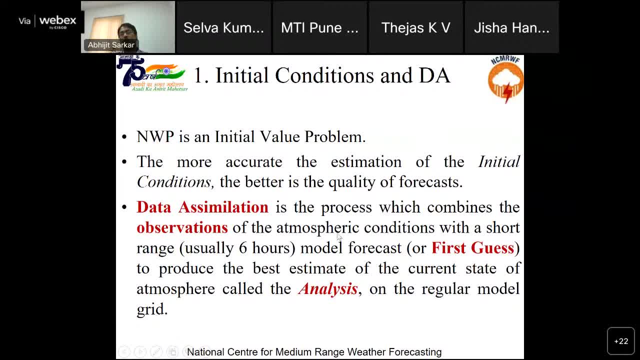 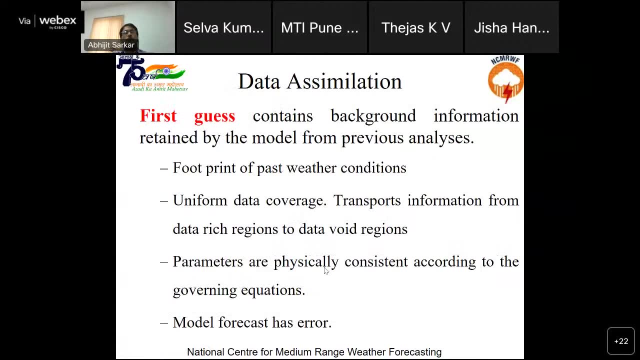 erroneous information, but both are valuable information. from these two informations we have to prepare the best estimate, the best estimated state of the atmosphere or analysis first case. first case contains the background information retained by the model from previous all the analysis steps so we can tell it is the footprint of past weather conditions. 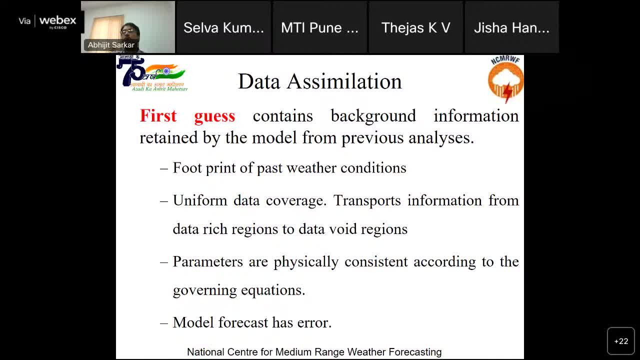 advantage of the first case is that it is data coverage is uniform. so what a regular grid at all the grid points. uniform data coverage is uniform. so what a regular grid at all the grid points. you will get the data, whereas observation is not available at all the grids. 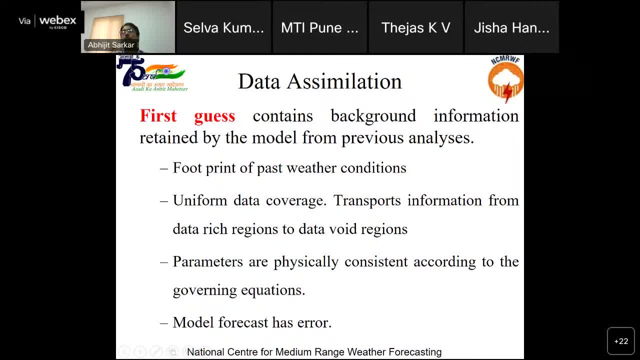 somewhere observator is very much irregularly spaced, it is not uniformly distributed. somewhere there are dents of the observations, somewhere the observations are very sparse. so what the model does? model takes the information from the observation, then when it runs, so finally forecast, it gives at all the gate points so we can tell the 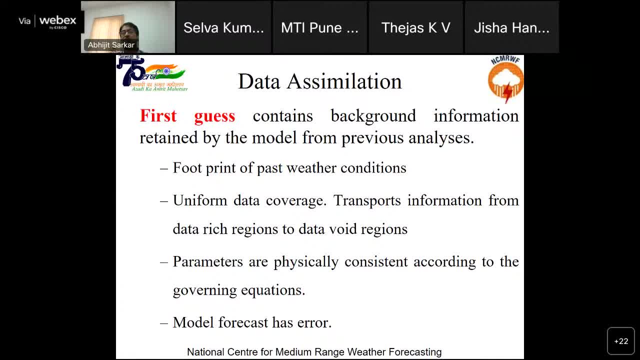 what the model does. it transports information from data to each region, to data by details. and since the model is formulated using the governing equations, so the model in the model output, the parameters are physically consistent according to the governing equations. so whatever the, we get in p in the model output, so the p is physically. 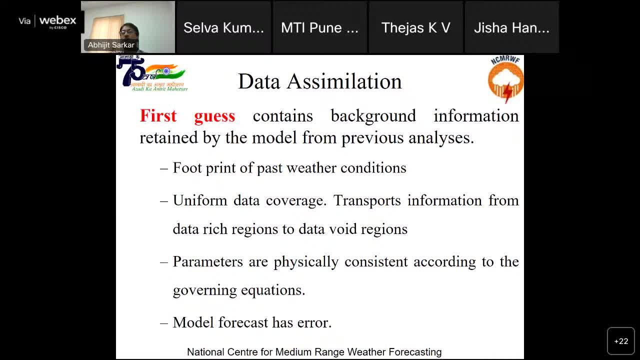 consistent with this u, v, q and t or these wind speed, specific humidity, temperature and pressure. all they all will be physically consistent with each other in the model output. but since it is a model, it is just one replica of the atmosphere, so the model forecast will have error. 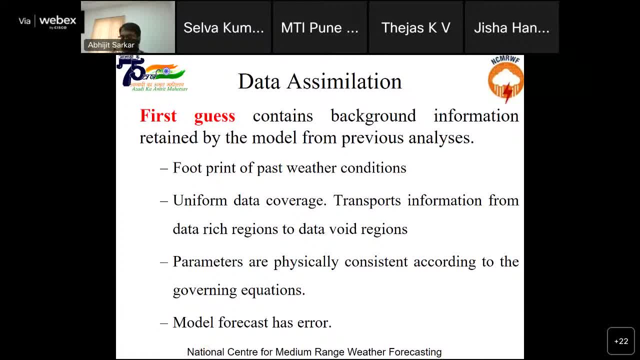 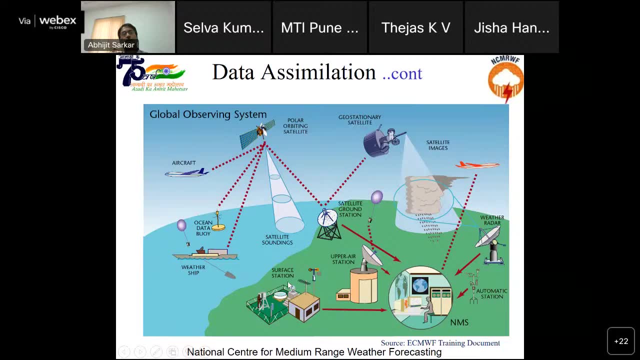 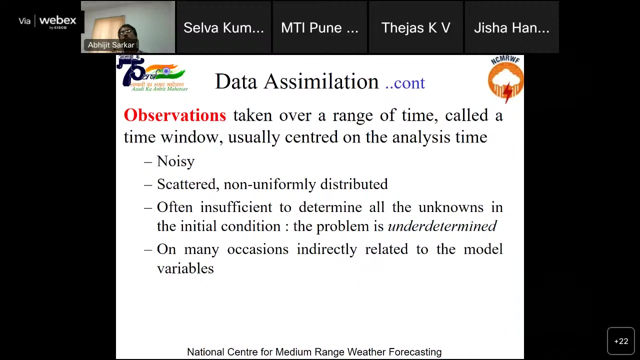 so we cannot tell. so it is whatever we get. we come to know from the model short forecast. so that is erroneous. so these are the sources of observations. the observation comes from air cap, from satellite, from radar, who we see, surface based observation observing stations. so from different sources we get observations. but the observations are also noisy, they have errors. 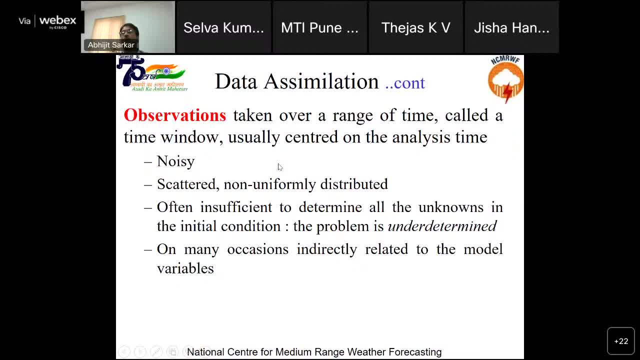 and, as I told, observations are not uniformly distributed. if you go to deep inside the sea or if you go to the himalayan region, so hardly we will get any observation. very small number of observations are available, but some other places a very dense population of observation. 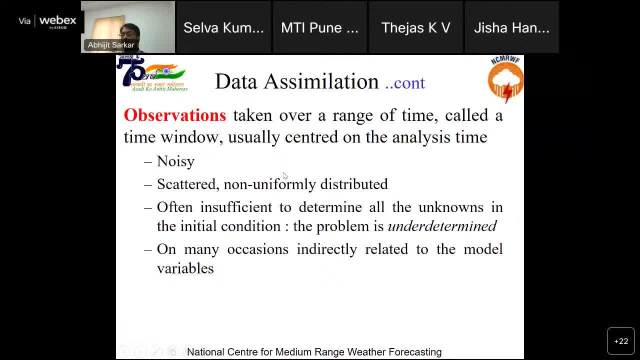 so if we need the data at about 10 to the power 13 or 10 to the power 14, 10 to the power 9. number of points observation: we get about 10 to the power 5 or 10 to the power 6. 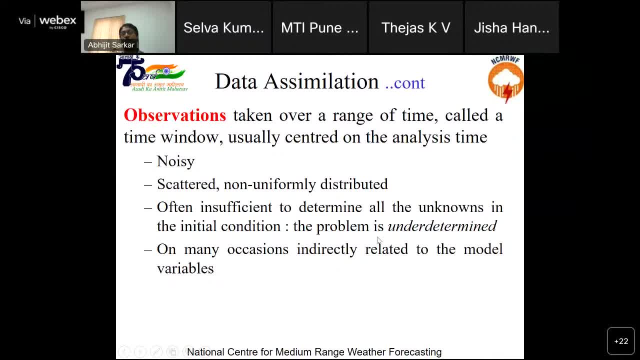 you can tell that observations, number of observations is insufficient. this problem is called undetermined and on many occasions indirectly related to the model variables. suppose the satellite observation. it does not give directly the temperature or humidity, it will give you radiance. so then, which forms, with some equations: 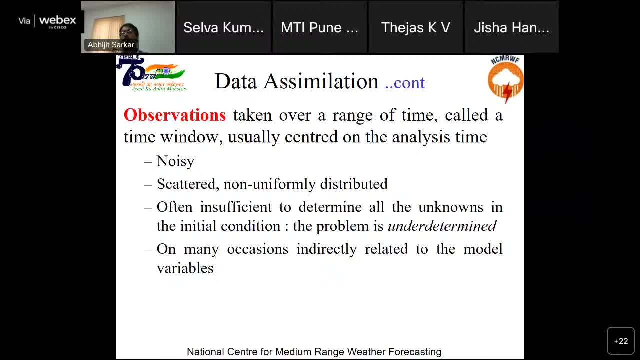 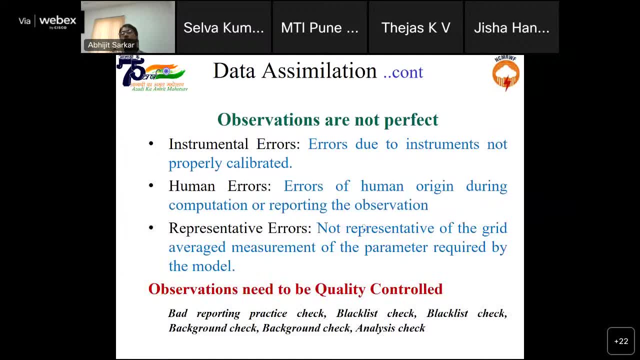 that humidity or the temperature will be converted into radiance. so they. what are the sources of these errors in the observation? first is instrumental errors, then human error, errors of human origin during computation or reporting the observation, and representative errors. we need the data at the model grid points and that data should. 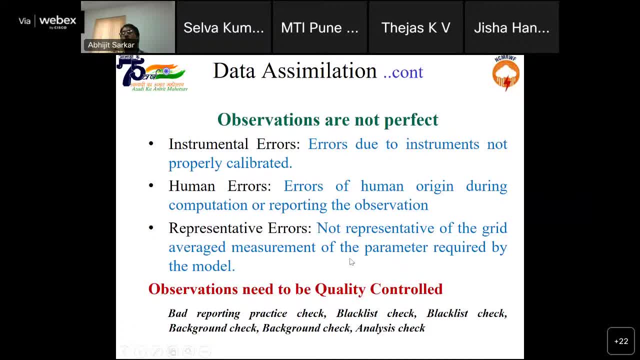 represent the grid average in value means what data we are giving at the model grid point. so that should represent the average over the whole grid box. but in observation we don't get that. we get a point: observation it is not the grid average in value. so it is not the fault of the. 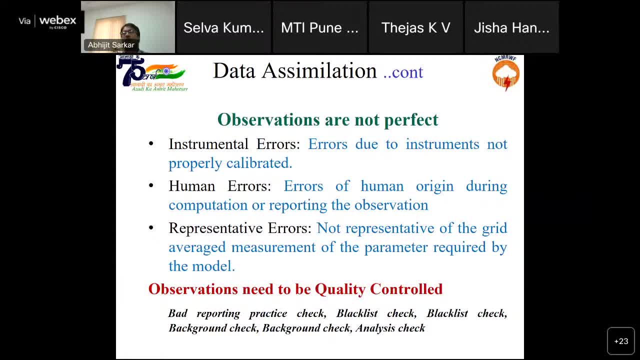 observation, but the error is attributed to the observation and it is called representative error. and because of these many errors the observations are required to be quality controlled. so we have to make bad reporting practice. check then some stations- they always give bad, always give erroneous observation. so you have to blacklist those stations, so you have to. 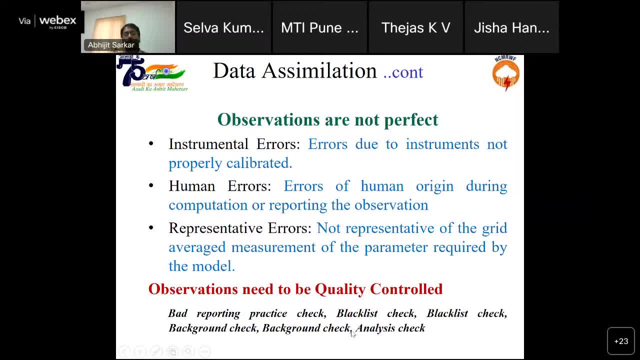 blacklist check. then we have to see the data, what i have received, whether they are close to the background background check and then analysis is checked. so different types of checks are there through which we can quality control the observations, since observations are valuable. we don't easily remove any observation. so till the 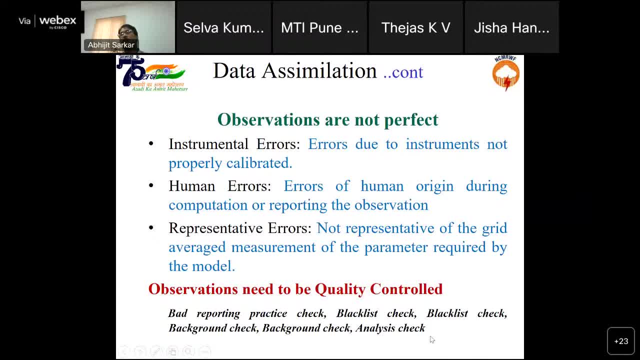 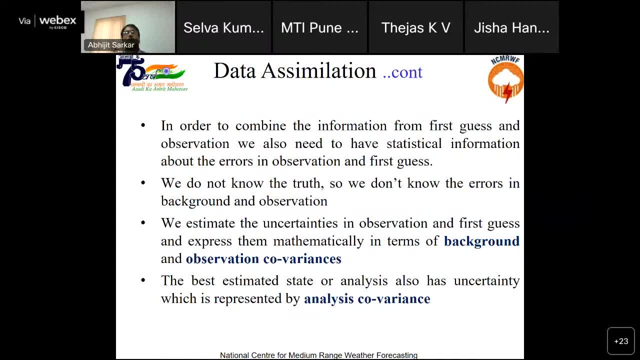 end that during the analysis also we check whether that observation can be accepted. in order to combine the information from the first case and the observation, we also need to have statistical information about the errors in the observation and first case. we know that these two informations have error and we don't know how much error is associated with an observation. 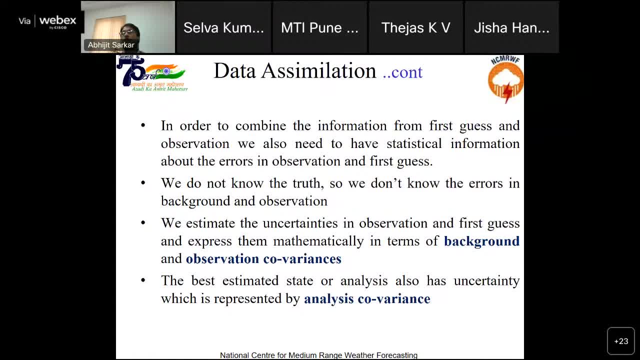 because we don't know the truth. but we have the error statistics and we don't know how much error is associated with an observation. so we can estimate the uncertainties in observation and fast guess and express them mathematically in terms of background and observation covariances. so background covariance: 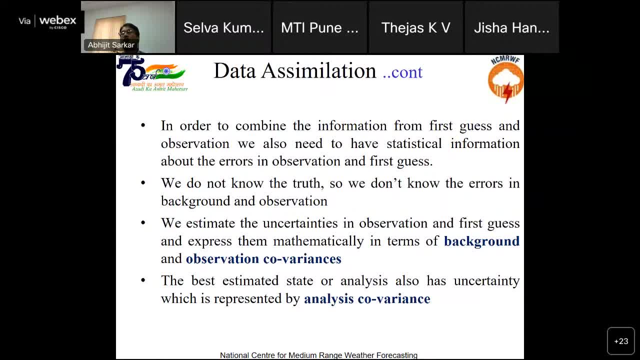 and observation covariance. they represent the uncertainties associated with the background and the observation. so we have four information. one is background or fast guess, another is observation, another is then background covariance, then observation covariance. on these four informations we try to prepare the analysis. we want to minimize the uncertainty in the initial state. so that means we want to. 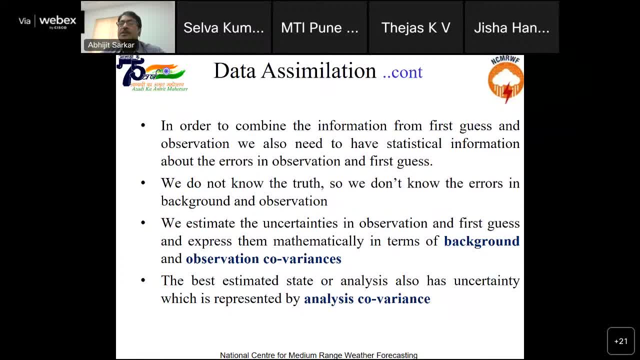 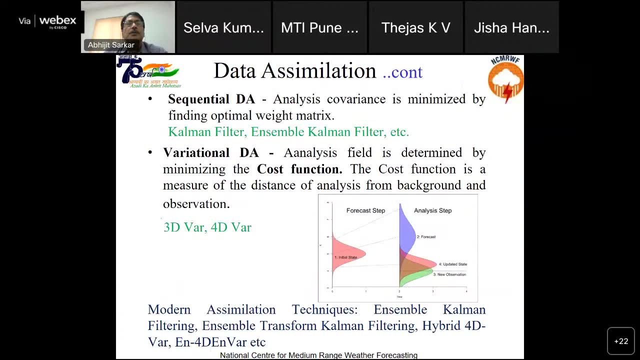 produce, or we want to generate, the best estimated state of the initial condition state of the atmosphere, but still it will have some error and that error will be represented by analysis covariance. there are different methods of data assimilation, but mainly two categories we can divide. one is sequential data assimilation. 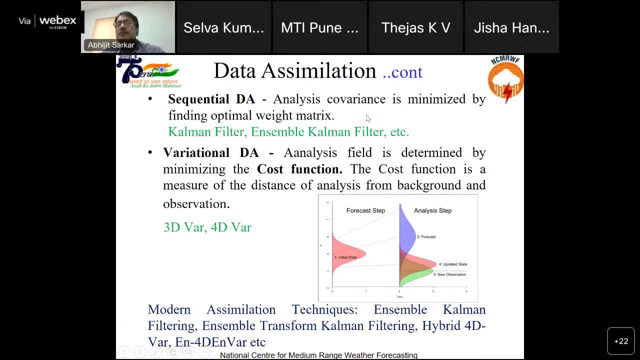 in this data assimilation method analysis, covariance is tried to be minimized by finding optical weight matrix. and in this data assimilation method analysis, covariance is tried to be minimized by finding optical weight matrix. the information which has less uncertainty that more weightage is given to that. 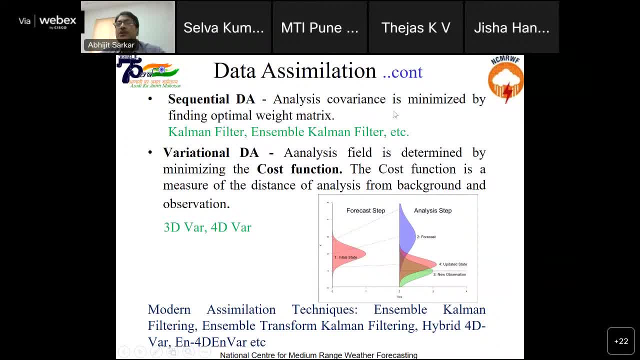 so in this sequential data assimilation system we calculate that weightage factor. so analysis covariance is minimized by finding optical weight matrix, and examples are kalman filter, ensemble kalman filter, extended kalman filter, etc. anyway, but that is it. as you see, in thegia we have created a followed line. 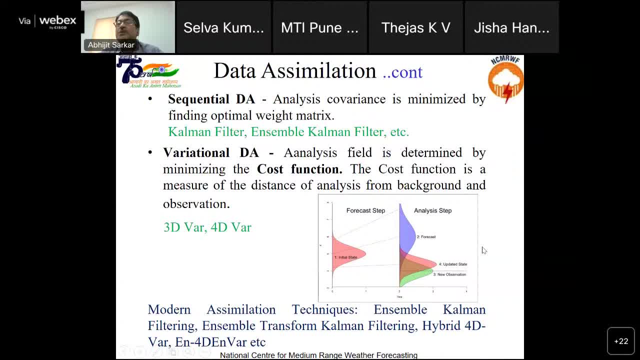 now what you can do is that i will run another K1 step, which are the best Things we can do. so, that is to say, we have produced some values which are very good, because this is basically taking the value of an association model we want to achieve. 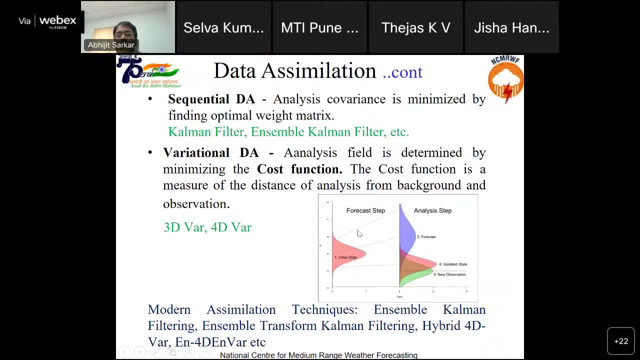 here one figure, so the two steps. here they are described. so if we have some initial state left side that uh pink color, if you can see this probability density function, so it is representing the initial state. so it is telling that in the initial state also there is some error. 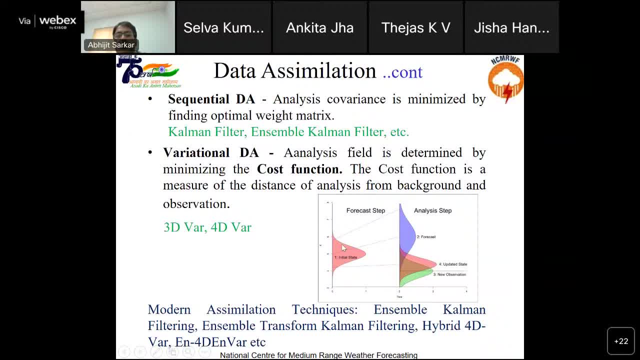 or uncertainty, because it has some finite variance or standard deviation. so now the with the help of the model, so it is. it is evolving, so that means we are giving the forecast so that error will grow with time. so after six hours that error has grown. so as a result, the variance has increased. 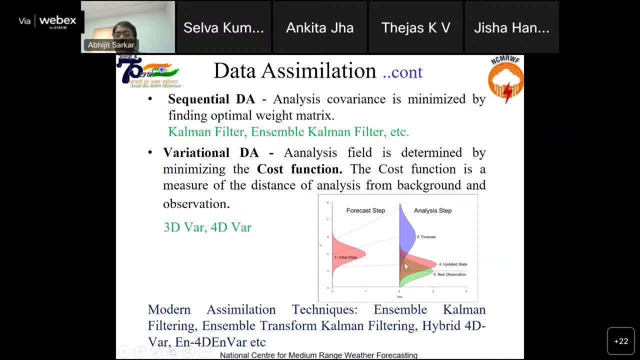 so we are getting probability, probability density function of the forecast. so this is our first guess: that blue color probability density function, and then again that pink color probability density function. oh sorry, this green color probability density function. it is giving our giving us the observation at that later time time. two observation also has some error. 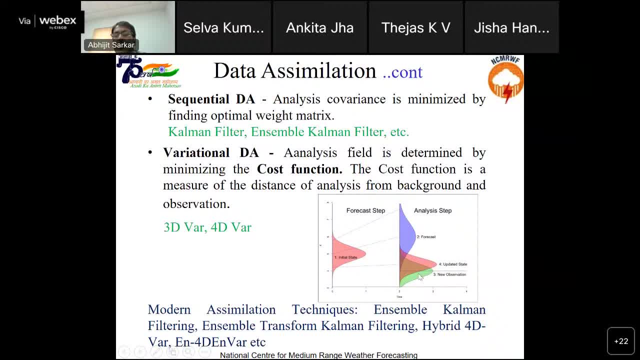 now the objective of the data assimilation system is to find out that best estimated state of the atmosphere or the analysis which will have the less uncertainty, less uncertainty than both their fastcase and the observation. so this pink one, pink probability density function will be the first good. then the next denotation process: available transportation trajectory to economic nation values have equal relative scale. that we expect it will not have any place. uncertainty, less uncertainty stack which will have�a osla value, Multiply regions, heating constant tasty, and this link as shown in the introduction here, this think inequalityolu Ojani, Puch, undeclared model isahi, given test will see which. 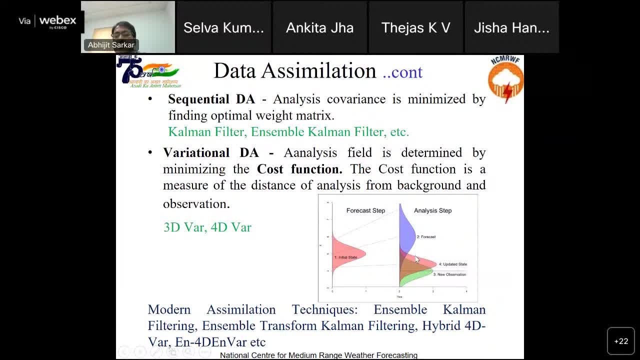 we will have lesser variance than that green and also the blue. And then modern assimilation techniques are: ensemble Kalman filtering, ensemble transform Kalman filtering, hybrid 4D VR method, ensemble 4D ensemble VR method, etc. So what we can understand, that, with the help of data assimilation, we are preparing the 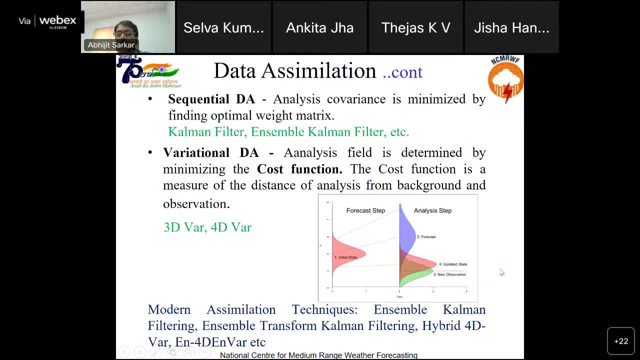 best estimated state of the atmosphere, but still that best estimate also will have some error. And at the end of this data assimilation method what we get? We get a physically consistent set of variables. That is very much essential For running the model. 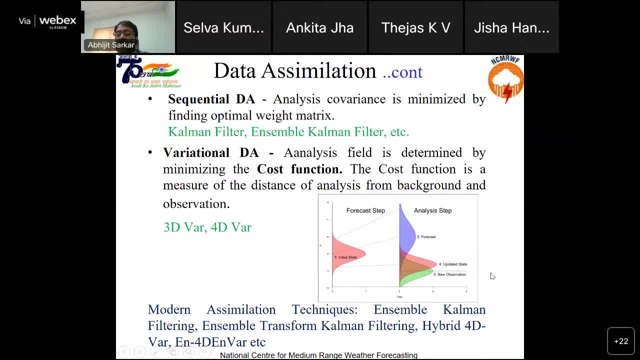 Because if these variables are not physically consistent with each other or initialized so, then some very high frequency, noises, gravity, inertia, gravity waves will be generated when the model will run, So with time, so those waves will dissipate, those waves will be dampened. 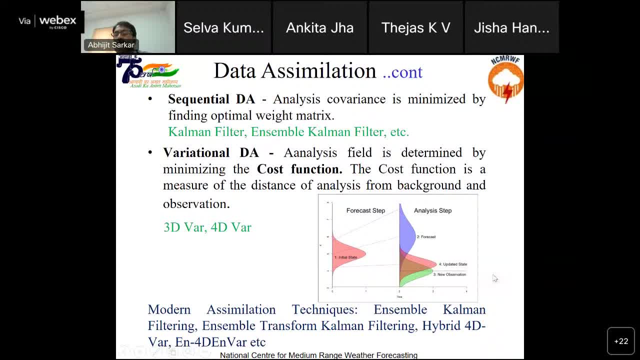 But it will take some time. So that time is called spin-up time. We don't a large spin-up time of our model because our the short-range forecast should be very accurate. If short-range forecast is not accurate, then our first guess will have a lot of error. 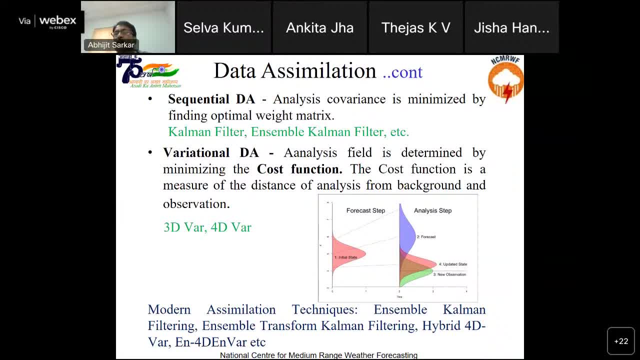 So to make our first guess correct, we have to remove these high frequency noises or we can tell that we have to make these variables physically consistent with each other. So now it is modern data assimilation methods, all the methods. So they make, they give us the physically consistent variables. 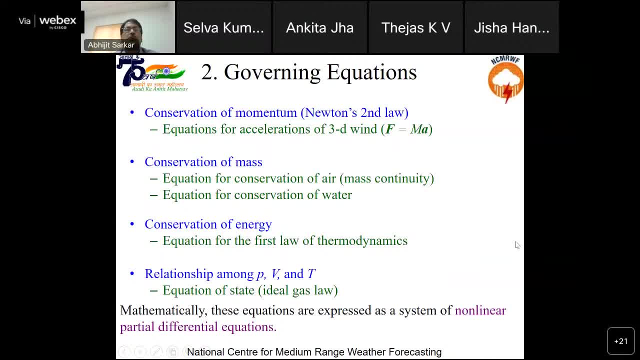 After this we have to formulate the governing equations, and governing equations include conservation of momentum equations, the three equations for accelerations- that means Newton's laws- then conservation of mass equation, one equation for air and another for water, that one separate conservation of equation for conservation of water is required. 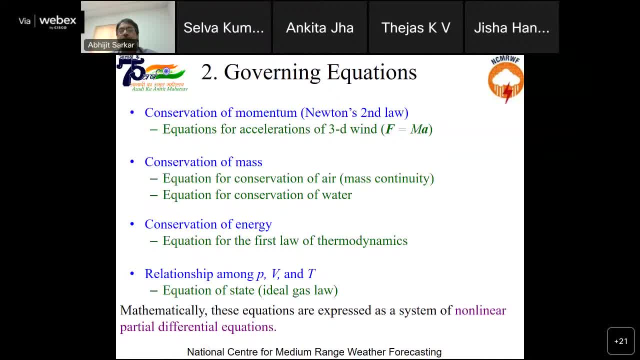 not only because precipitation is very important, But also that water is the main agency which transports energy and moisture from one level of the atmosphere to another level. Then conservation of energy equation, or first law of thermodynamics, and the relationship among PV and T, that is, equation of state or ideal gas law. 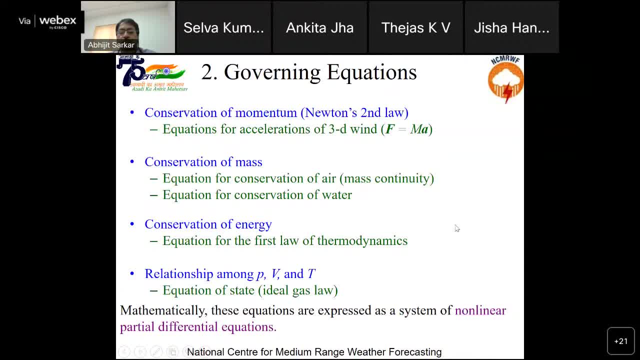 But all these Equations are non-linear, partial differential equations, so that means they have terms which is product of two dependent variables, that is advection term. So if not only these equations are non-linear, partial differential equations, they are non-linear. 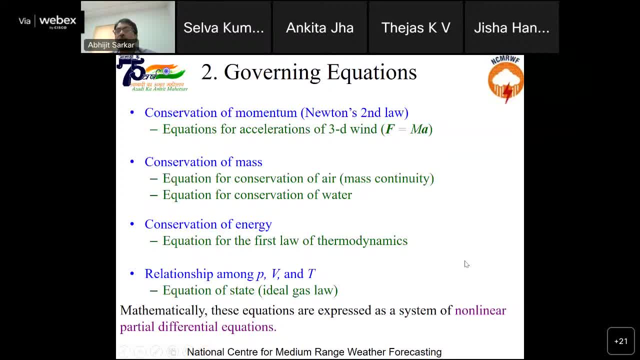 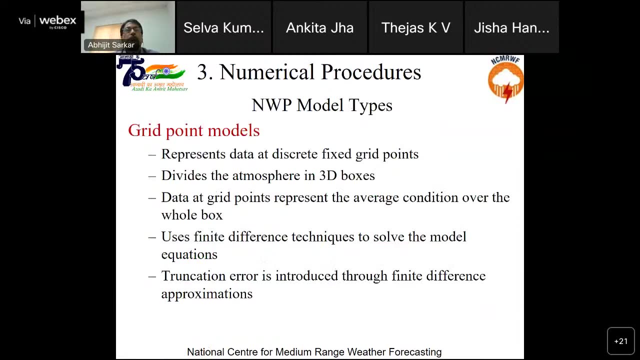 partial differential equations. So that means we cannot solve them analytically. so that means we will not be able to get that accurate solution of these equations. So we have to solve these equations numerically. There are two types of models. One is grid point model and the other is spectral model. 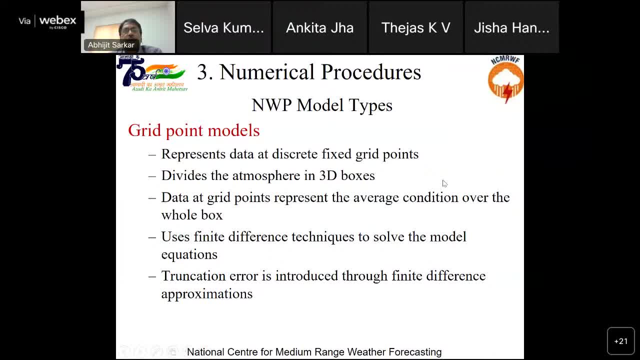 The grid point model divides the atmosphere in 3D boxes and data at grid points represent the average condition over the whole box. So at a particular grid point, if you get this temperature is 30 degree centigrade, it does not mean that 30 degree centigrade is not the average temperature. 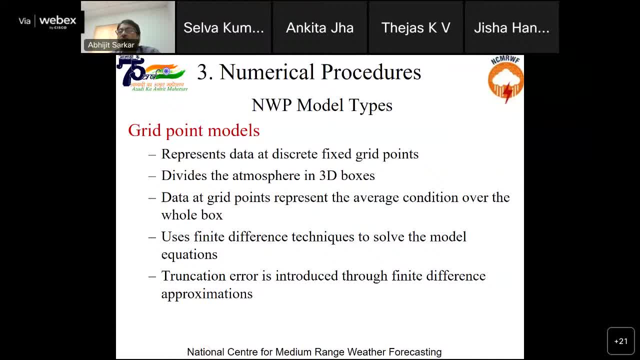 So at a particular grid point, if you get this, temperature is 30 degree centigrade, it does not mean that 30 degree centigrade will be at that location. It means that 30 degree centigrade is the average temperature over the whole grid box. 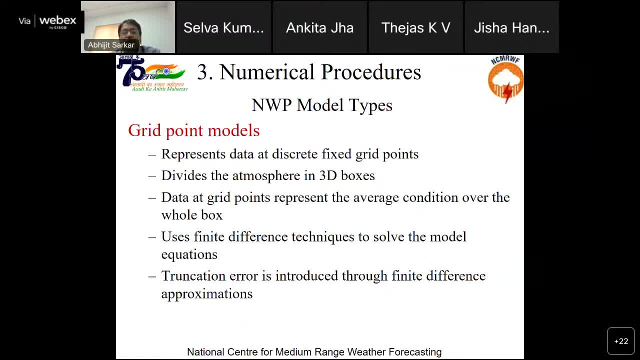 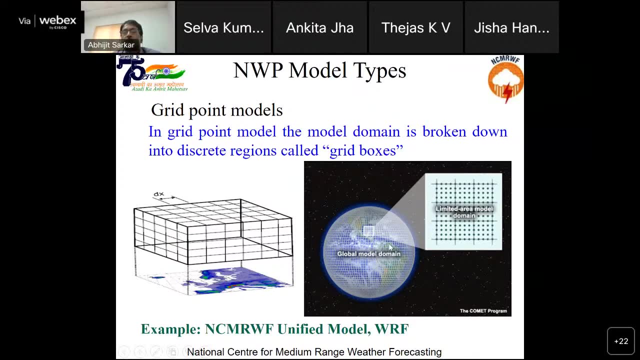 In the grid point model uses finite difference techniques to solve the model equations and truncation error is introduced through finite difference approximations So we can see the figures. So this distance between these two grid points, so we are telling it is dx, so a continuous 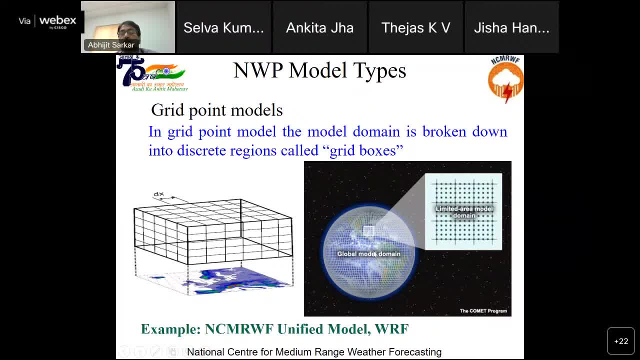 atmosphere is discretized, When the model covers the whole globe or it covers the atmosphere over the whole globe, so then we call it is global model. but because of the limitation of our computational resources we cannot always run these global models. If we want to study a very small system like thunderstorm, so then a regional model is. 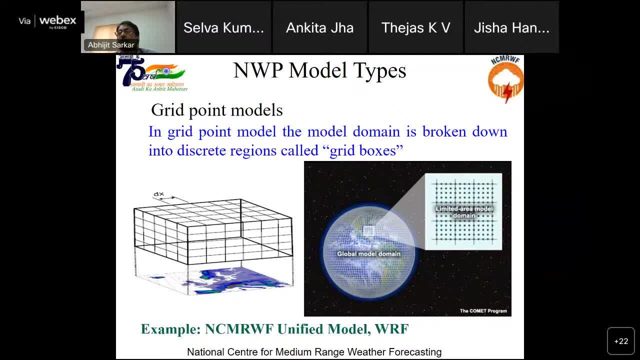 sufficient because we need high resolution. So with that high resolution, a global model will demand a lot of computational resources, So better to use one limited resolution. So this is the grid point model, and this is the grid point model and this is the. 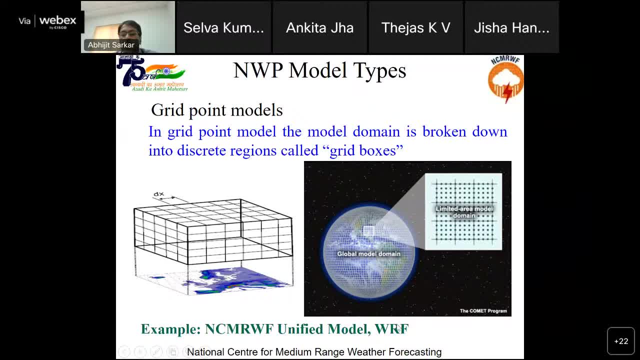 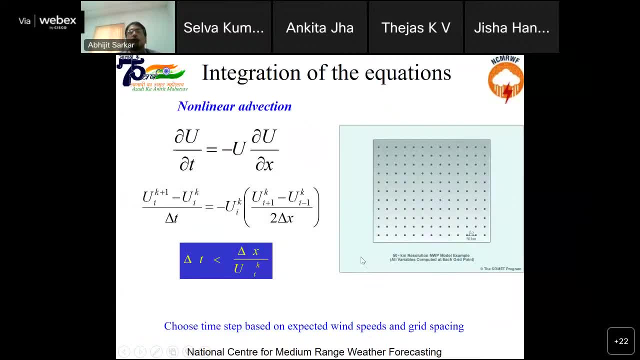 grid point model. The example of this grid point model is NCMRW unified model, WRF model, weather research and forecasting model. So these are the grid point models. So this is, you can see this equation, advection equation, which is taking the advection only. 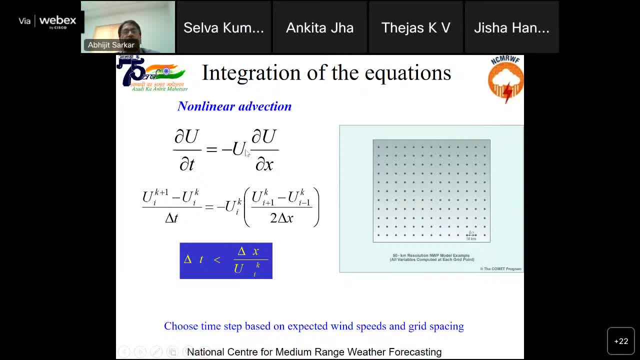 in the x direction, So right side. this advection term, This is: it is the product of two terms, two variables. One is u, another is del, u, del x. So these two are it is the product of two dependent variables. 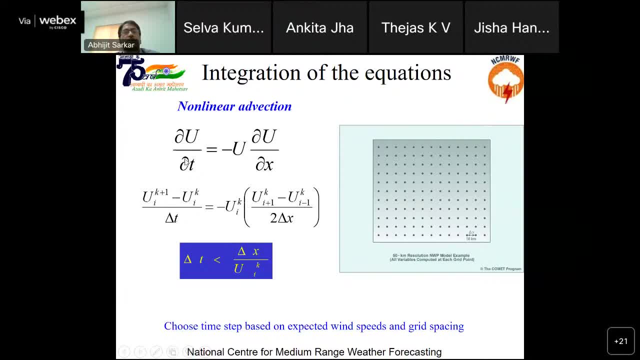 So it is a nonlinear equation. So we have to convert this nonlinear equation, differential equation, into a difference equation. So we are writing in this way That ui k plus 1. Minus ui k, where k is representing the time and the i is representing the space. 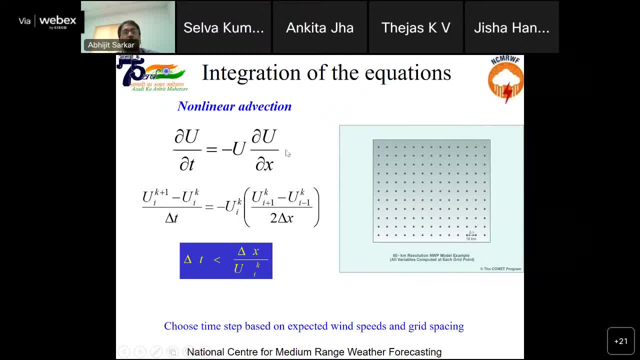 So we can tell, we are converting one problem of calculus into the problem of algebra By neglecting the higher order terms of Taylor series. So there will be some error. And one thing I forgot: That when we are formulating, When we are formulating the governing equations, 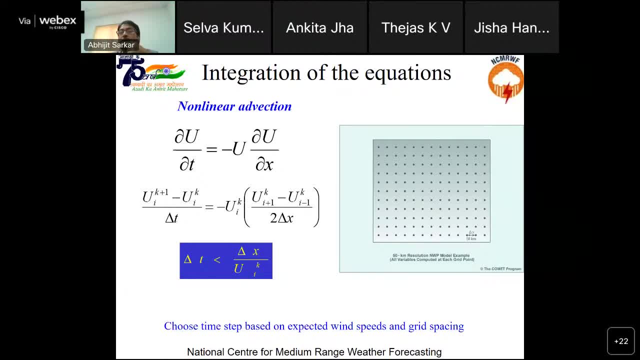 So we make several approximations And we neglect some terms which are not meteorologically significant And we want to remove actually very high frequency waves very fast, waves like sound waves. So we make some assumptions and we make some approximations, So there will be some error in formulating the governing equation. 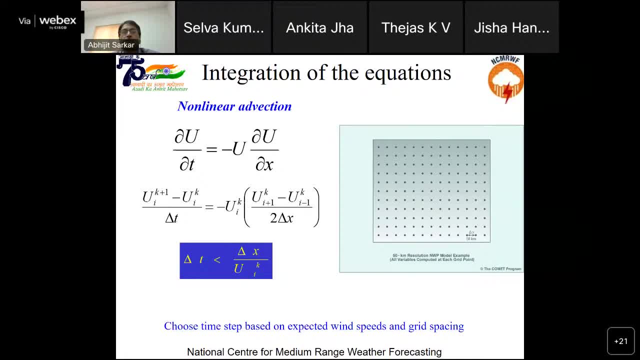 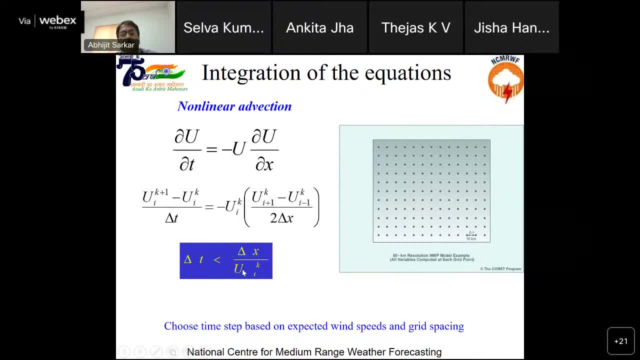 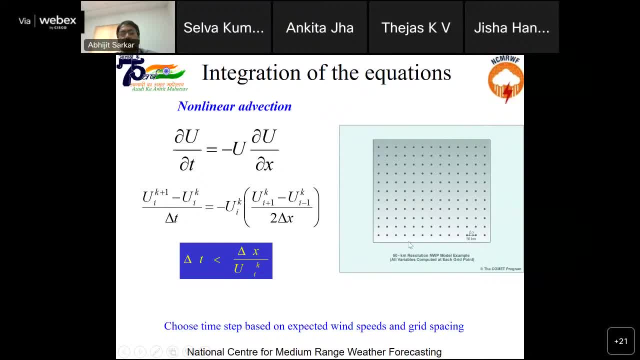 be very small and if you take a very high resolution model, so then its time step also will be very small. so that means you need more computational resources or 24, 24 hour forecast. you have to integrate over a larger number of time steps. so right side it is showing that what is delta x? so this is called horizontal resolution. 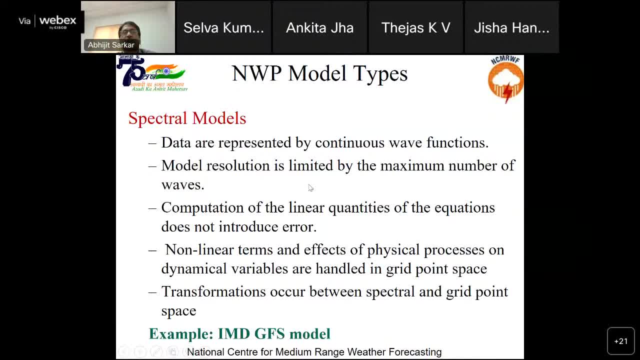 then spectral model. in spectral model, data are represented by continuous wave functions and model resolution is limited by the maximum number of waves. in spectral model, the linear quantities of the equations are computed in the spectral mode and non-linear terms and effects of physical processes on dynamical variables variables. 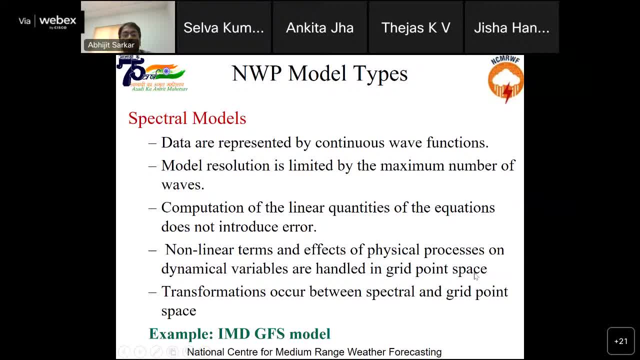 are handled in grid point space. But you have to always transform from the spectral or spectral mode to the grid model, grid point model and from the grid point model to the spectral space. But example of the spectral model is IMD, GFS model, then ECMWF global model. so that is. 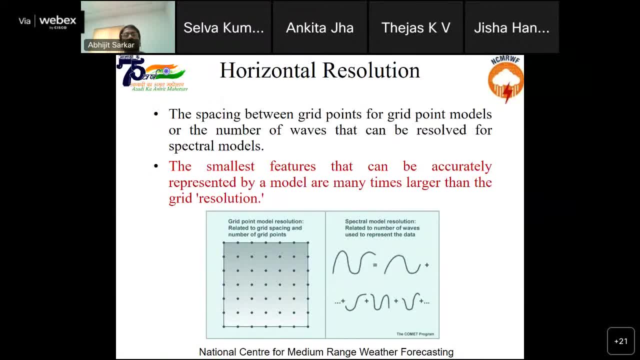 also spectral model. The horizontal resolution is the spacing between grid points- horizontal grid points in case of grid point model and the number of waves that can be resolved in case of spectral models. But the smallest features that can be added, accurately represented by a model, are many times larger than the grid resolution. It 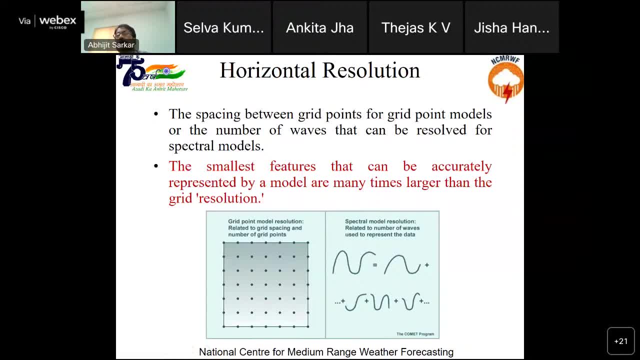 means if my grid resolution is 10 km, so I cannot resolve a phenomenon which extends to 10 km, because two grid points are not sufficient to resolve that phenomenon. So at least the number of waves that I want to resolve will be 5 or 6 grid points large. So then, only we. 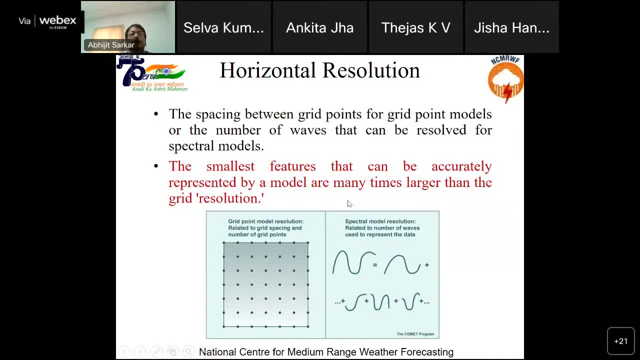 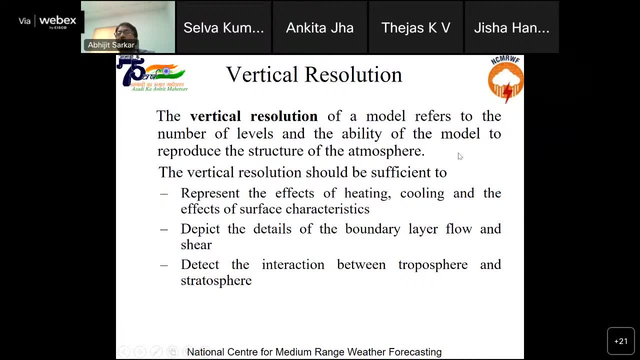 can resolve that phenomenon, Then vertical resolution of a model refers to the number of levels and the ability of the model to reproduce the structure of the atmosphere. So the vertical resolution should be sufficient to represent the effects of heating, cooling and the effect of surface characteristics So close to the earth's surface. the vertical 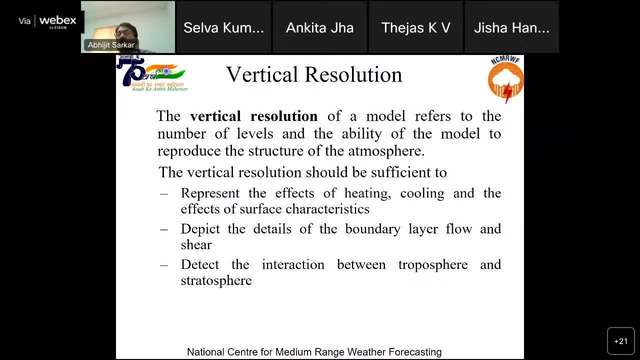 resolution should be very high, So where the distance between the vertical levels should be small, because here the gradient of the atmospheric variables, so this is very sharp, And again sharp gradient is noted between the near the tropopoles. So in a model it 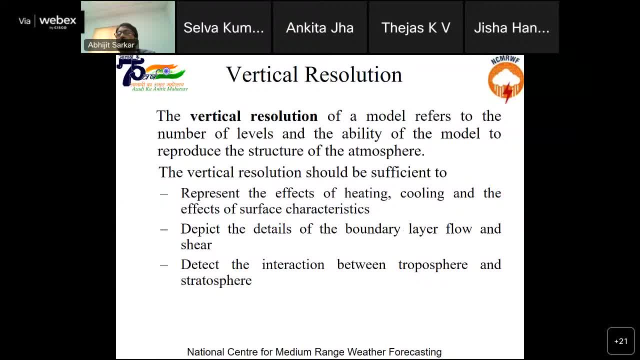 should be very sharp. And again sharp gradient is noted between the near the tropopoles. So in a model it should be very sharp. And again sharp gradient is noted between the near the tropopoles. So in a model 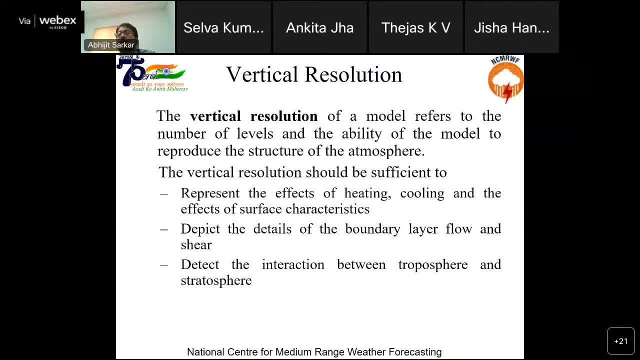 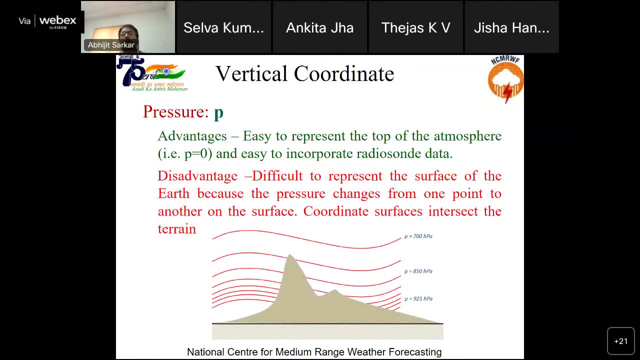 the number of levels near the tropopoles also should be high. Depict the details of the boundary layer, flow and shear, and detect the interaction between troposphere and stratosphere. What we should use as the vertical coordinate In the initial stage of NWP? the vertical coordinate. 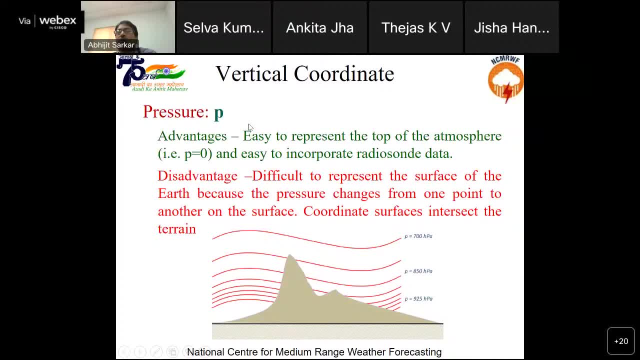 used to be used as the vertical coordinate, But there are some disadvantages of using this pressure as a vertical coordinate. Advantage is that it is easy to represent the top of the atmosphere and easy to incorporate radius on the data. A disadvantage is that difficult to represent the surface of the earth because the pressure changes from one point to another. 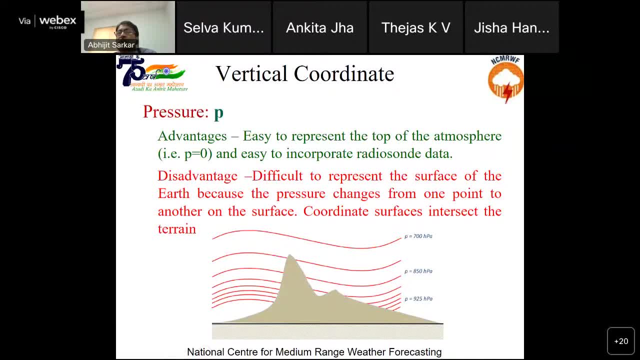 on the surface At all point. on the surface you will not get a particular value of p, a constant value of p. p changes over the surface. Over the mountainous region, p will be less, surface pressure will be small and over this plain region, the surface pressure 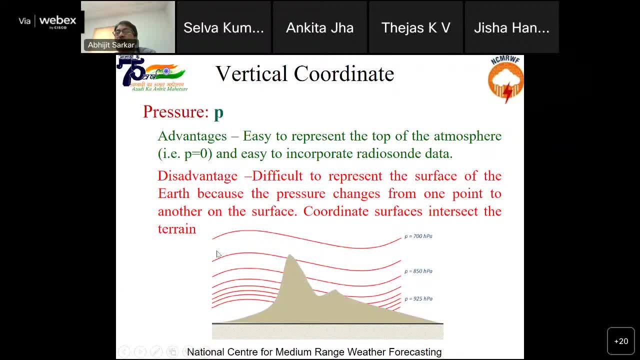 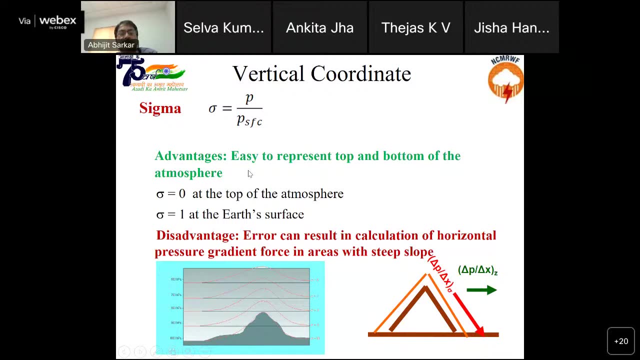 will be small And the coordinate surfaces intersect the terrain. Constant p surface, so that will intersect the terrain. So this is the disadvantage. Then sigma coordinate also can be used as a vertical coordinate. It has advantage that it follows the terrain. It is easy to represent top and bottom of the atmosphere You take. 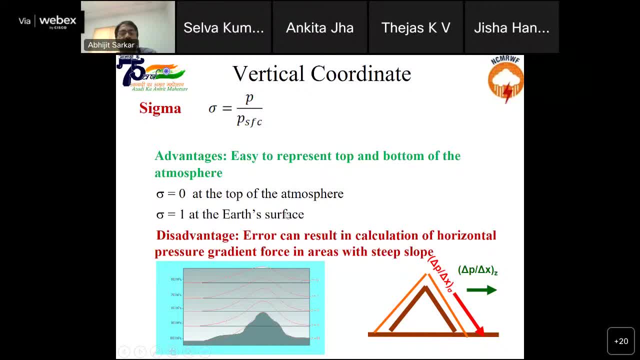 sigma is equal to zero at the top of the atmosphere and sigma is equal to one at the earth surface. So we are getting a constant value of sigma at the lower boundary as well as at the top boundary. But main disadvantage is that pressure gradient term you cannot calculate accurately at sigma. 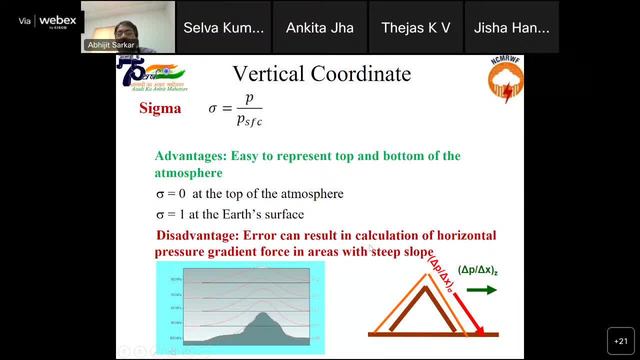 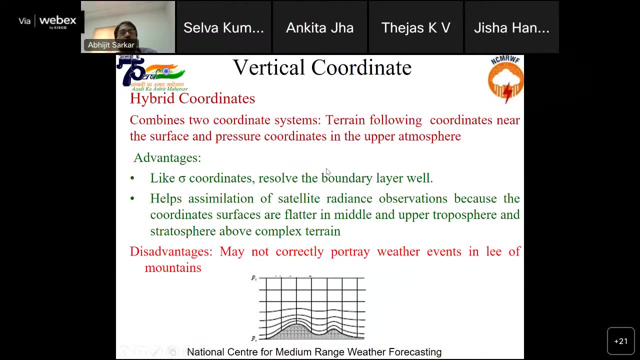 coordinate system Error can result in calculation of horizontal pressure gradient force in areas with steep slope. So in the modern NWP systems that hybrid coordinate system is used as a vertical coordinate. So it is the combines two coordinate system: terrain following coordinate coordinates near the surface and pressure coordinates in the upper 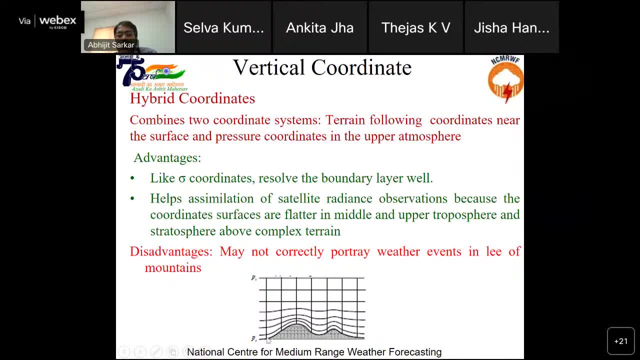 atmosphere, So that the near the surface it follows the terrain and as you will go up so it becomes flat. So it is flattenedность道, Assgun the said myth by spiral. Its disadvantage: It may not correctly portray whether it bends in the lee side of the mountain. Focus attention to the 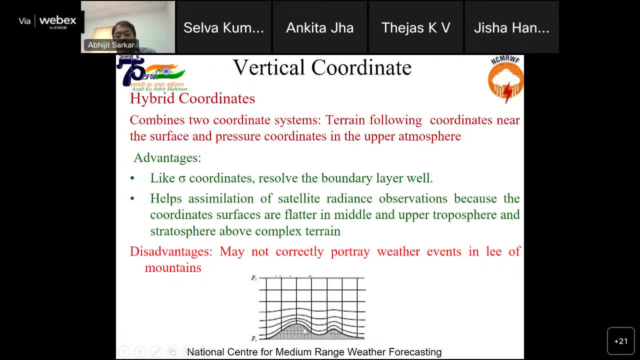 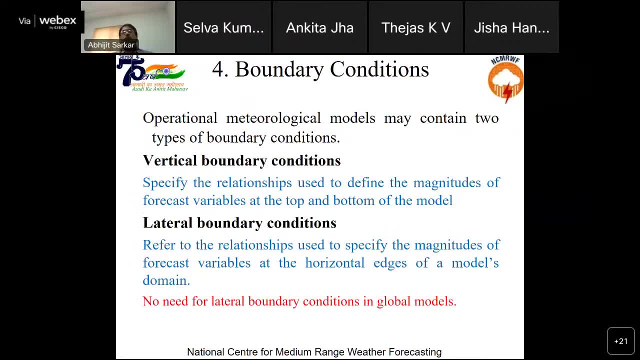 is what the disadvantage of sigma coordinates, so that can be seen here also. Then comes boundary condition. In our actual atmosphere there is only one boundary, That is Earth surface. They alleways In the sailing surface, they all unique to one boundary. Through the Amazing Project by가정, We all will see again. That is what this entire thing is about. Like the accident is 허� 아이라 as the after Stevens, It will all sitter alive in the sun, though it touches there for two hours. 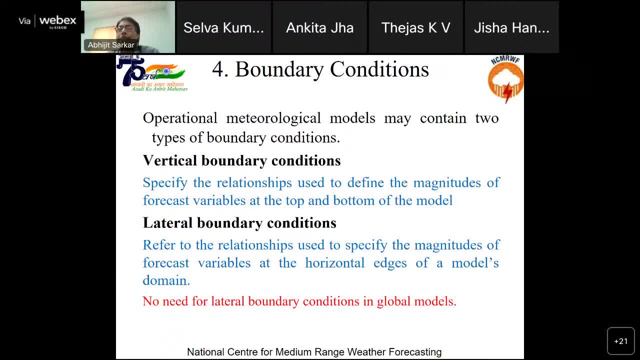 That is the Def Monkey and before, And they are two denke to remind you that they all are not active for auur later. it is the first crossing by earth surface. But in a global model we need two boundaries. We have to incorporate one. 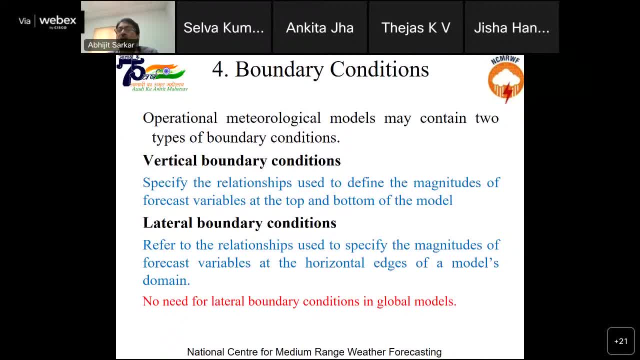 artificial top boundary also. Otherwise our calculation will not be complete, It will never end, But we have to give the forecast within a stipulated time, So we have to artificially fix some top boundary. In our NCM-RWF global model the top boundary is at 80 kilometer height. 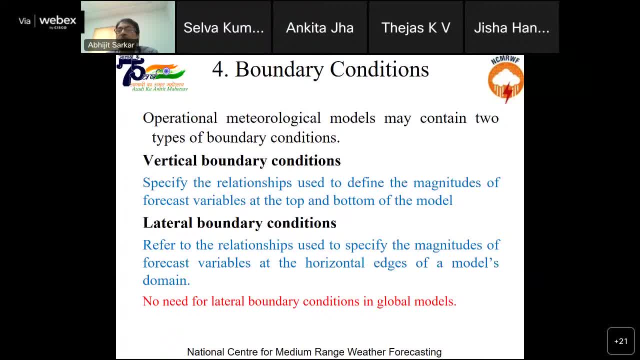 In our regional model the top boundary is at 38.5 kilometer height And in a regional model, so again four more artificial lateral boundaries. we have to fix These vertical boundary conditions that specify the relationships used to define the magnitudes of forecast variables at the top and bottom of the model. 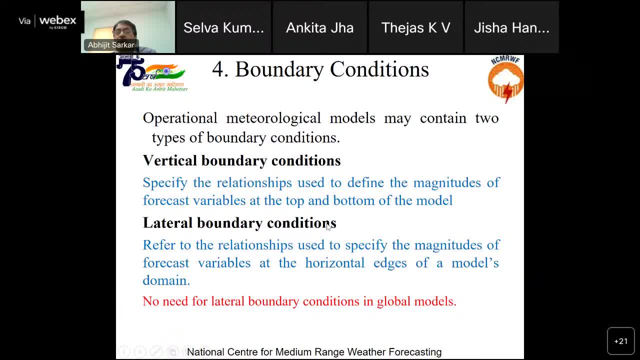 And the lateral boundary condition means the four side walls of the limited area model. It refers to the relationship used to specify the magnitudes of forecast variable at the horizontal edges of a model's domain, And the lateral boundary condition means the four side walls of the. 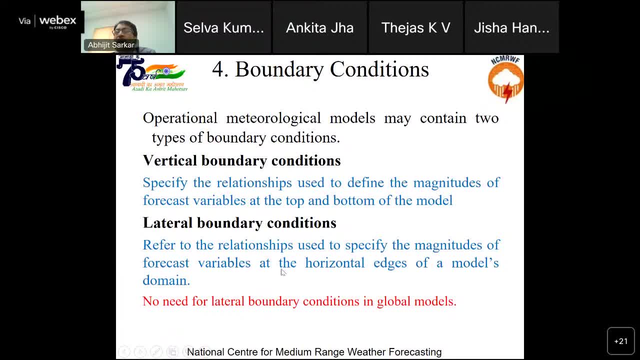 So we have to specify the values of the variables at these boundaries. When the model is running, the information is passing from one grid box to another grid box. For the interior grid box, it is okay. That information is passing from one grid box to another grid box in the form of the equation: 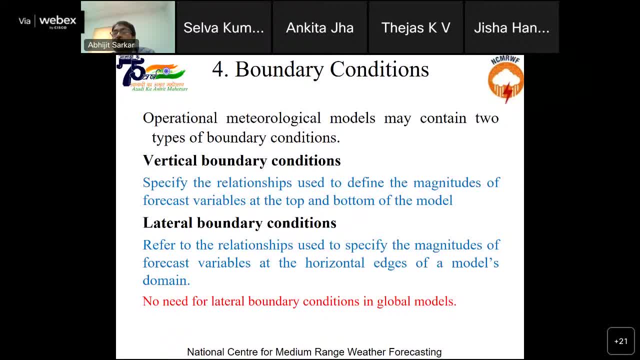 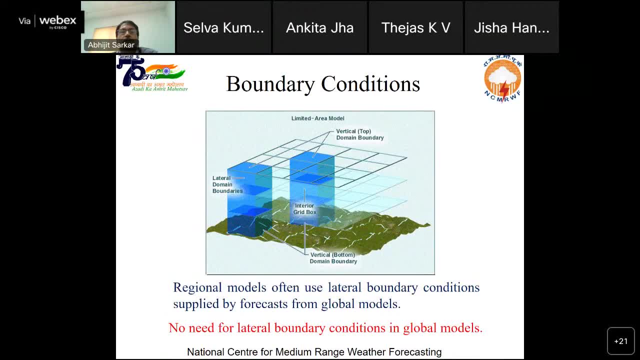 But at the edge, at the boundary, we have to provide that information So we can see: this, is this, these interior grid points. So from one box to another box, the information is can pass in the form. these are in the form of advection term or the diffusion term. 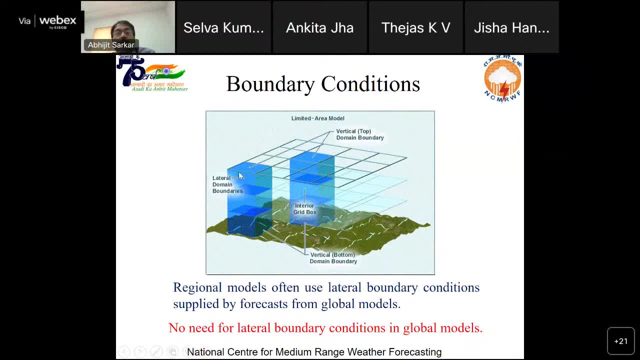 But when the point is at the boundary. so then you have to provide the information For the, for the regional model, the lateral boundary condition it gets from the global model forecast And in the lower boundary. so this we have to give, some bottom boundary conditions We have to provide. 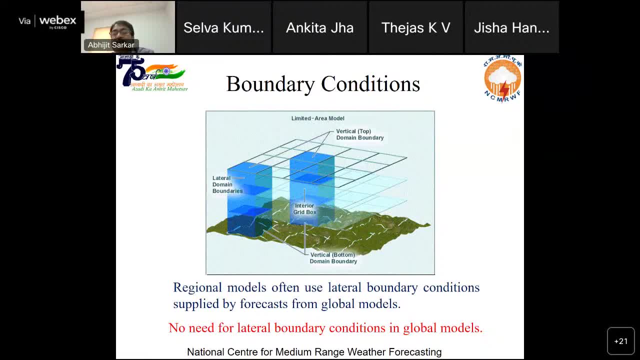 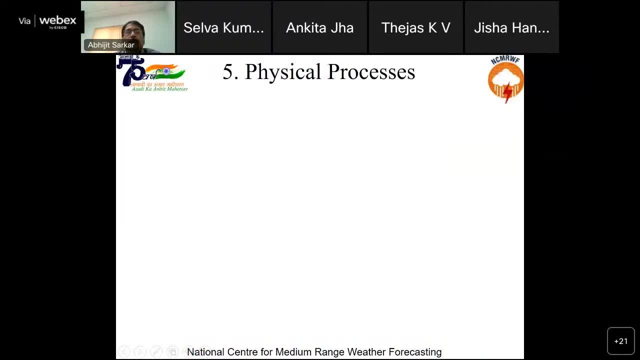 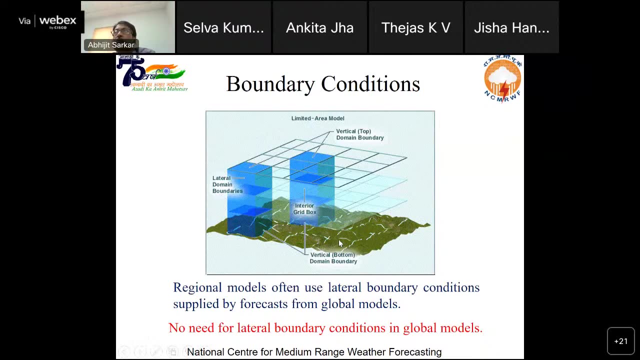 the topography, landings and so on. So the topography is given by the lower boundary conditions. So the topography is given by the ground, boundary conditions, the elevation conditions, land cover, vegetation, all the surface parameters. So, but because of the finite resolution of the model, 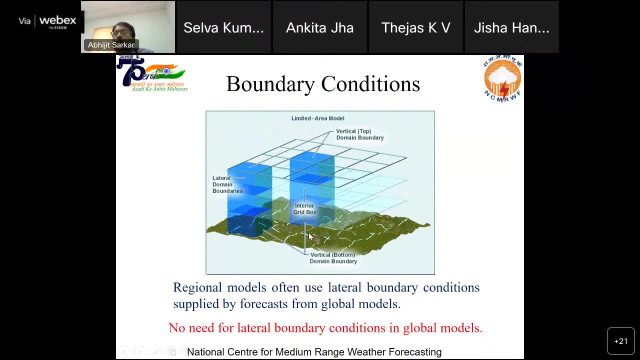 we cannot provide the every detail of the lower boundary. If my model resolution is 12 kilometer, so within the 12 kilometer distance the non-homogeneity of the surface or non-homogeneity of the lower boundary we cannot specify in the model. So that is a problem. And again at the lateral boundary, 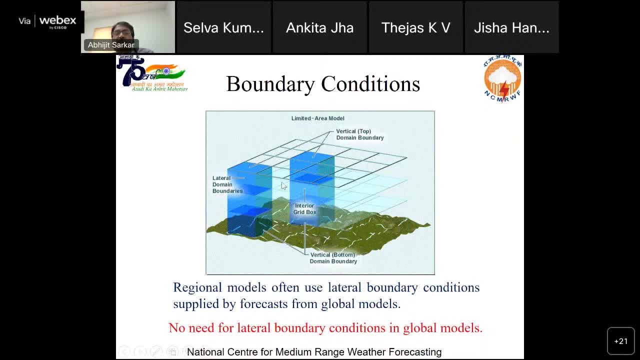 we can give this input or we can specify the boundary condition only at final need. Thank you, Thank you. So within this three-hour time we have to interpolate the boundary condition to get the value at every one minute. So there will be error in specifying the lateral boundary. 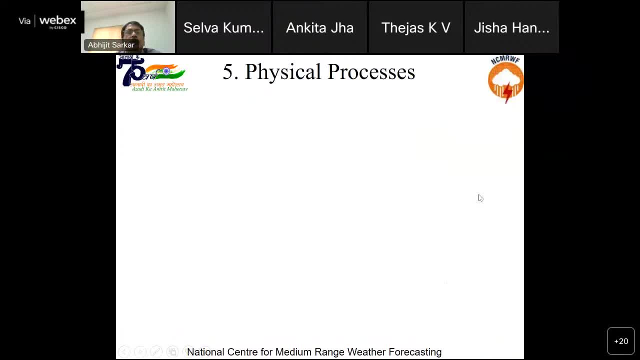 condition also. Next comes physical processes. So there are small-scale processes which are very important. The effect of these processes are very significant in the large scale but because of the finite resolution of the model we cannot resolve those processes. So these processes are called. 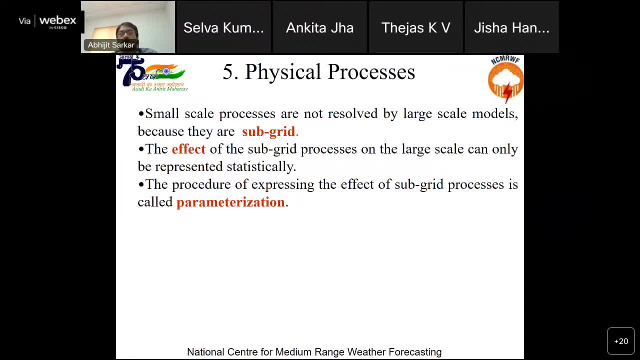 subgrid-scale processes. Although these processes are very small, their effect is significant in the large scale. So unless we take into account of the effect of these processes, our model forecast will not be good. The procedure of expressing the effect of subgrid-scale processes is called. 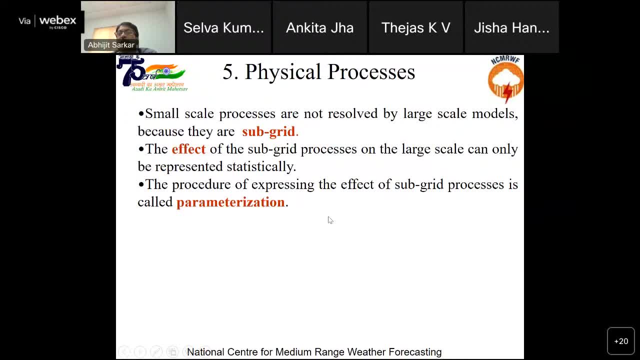 parameterization. So we take into account of those processes, with some assumptions or approximations, or statistically. So somehow we have to take into consideration the effect of these processes. So we have to take into account the effect of these processes. So 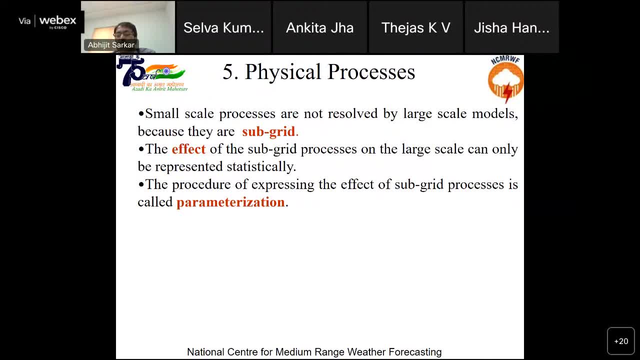 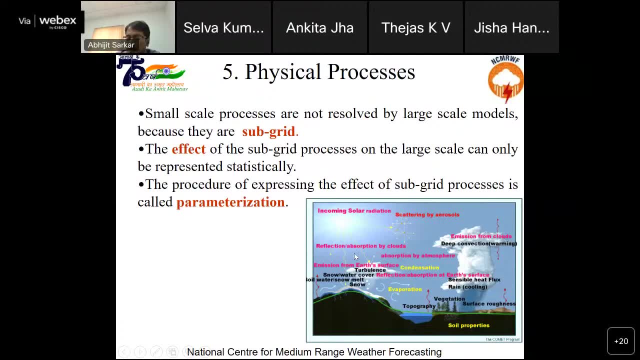 thisigerłączung, that is the demonic. here is an equivalent of physical processes, where all of the various physical processes are account for a significant effect of these small-scale processes. So these are the different physical processes, that which we have to consider within our model, like radiation transfer, surface process, vertical, turbulent process. 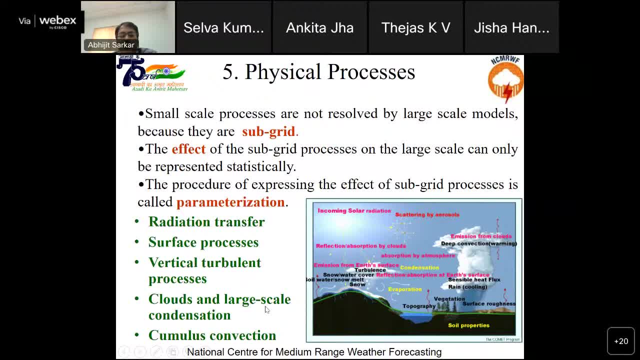 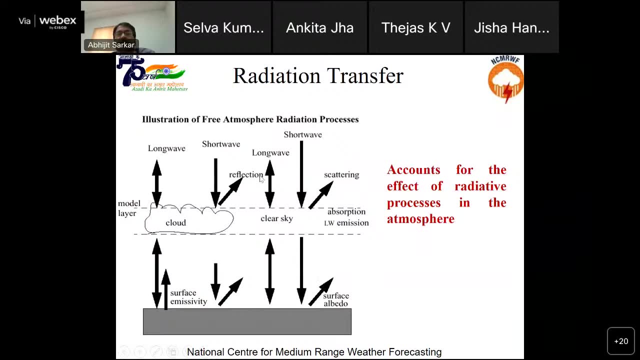 clouds and large-scale condensation cumulus convection. So, very briefly, I will talk about these processes one after the other for the next steps. So we have taken some some very simple after another. what are these processes? first is radiation transfer, so these processed accounts. 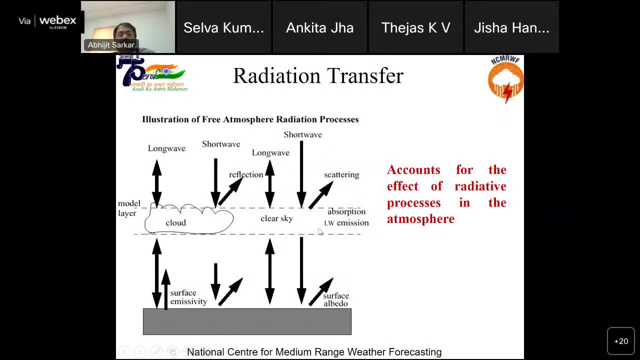 for the effect of radiative process in the atmosphere. so that means how much long wave radiation is going back, how much short wave radiation is coming to the atmosphere from Sun, how much? what part is reflected back by the cloud or albedo then? so all these things are taken into account in these processes then. 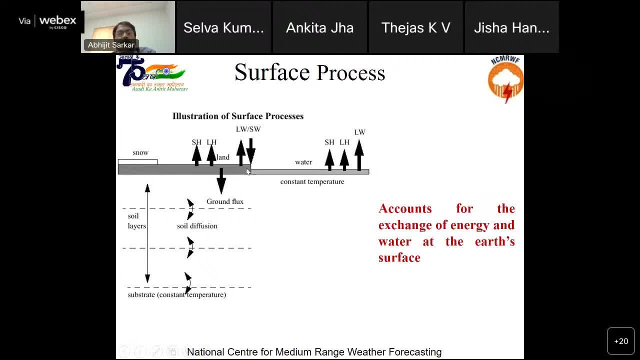 surface processes. so this process takes into account the exchange of energy and water at the Earth's surface. so how? what is this? how much is the sensible heat flux or latent heat flux from the land? or long wave, short wave radiation? what is long wave? how much long wave radiation is going away? 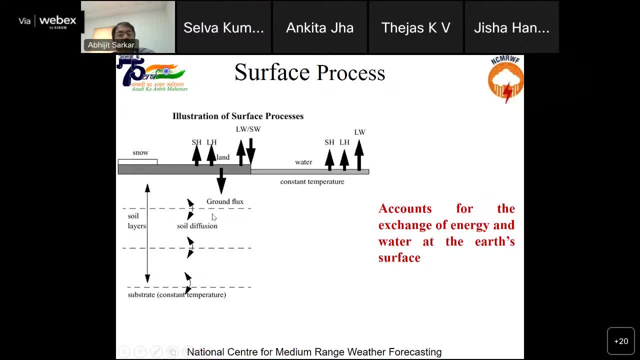 how much short wave radiation is coming, how much part is going to the ground and how much is refused to two different soil layers. so there will be inhomogeneity over the lower boundary layer, lower boundary also. so there, somewhere there will be snow, somewhere there will be water if the surface characteristic changes this. 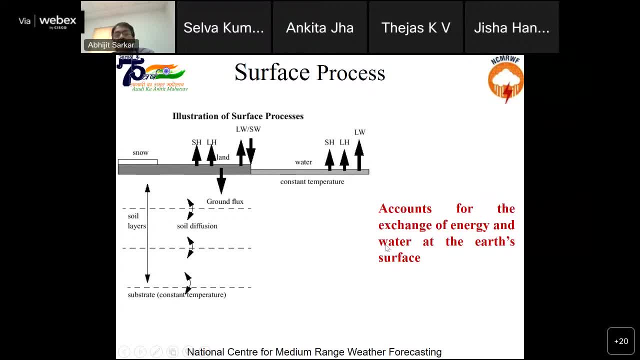 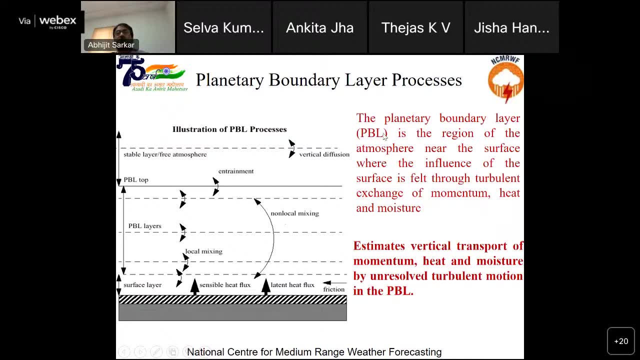 processes also will change. so those things will be taken at taken into account in surface process. then comes planetary boundary layer process. now, the planetary boundary layer is the region of the atmosphere near the surface where the influence of the surface is failed through turbulent exchange of momentum, heat and moisture. 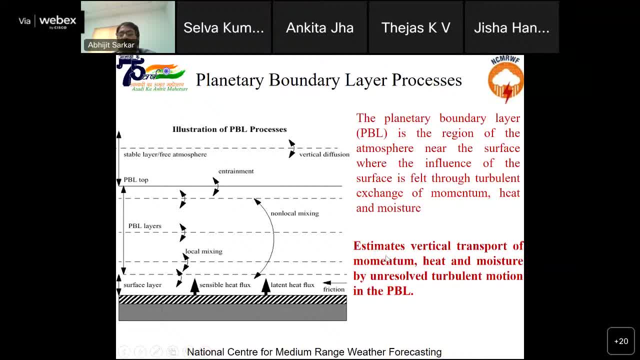 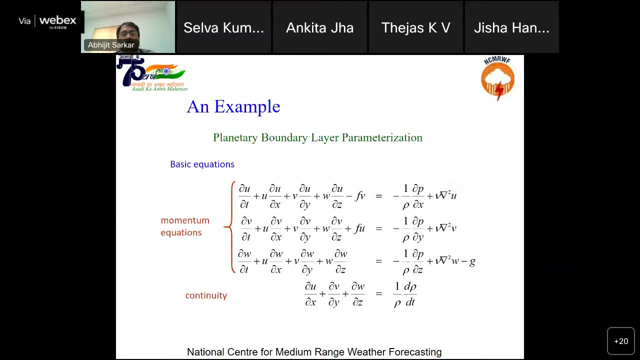 it estimates this PBL process. it estimates the particle transport of momentum, heat and moisture by undissolved turbulent function in the PPL. so how do we do parameterization? so, with the help of a very simple example, so I will show this how we do the, how we parameterize this PBL process. 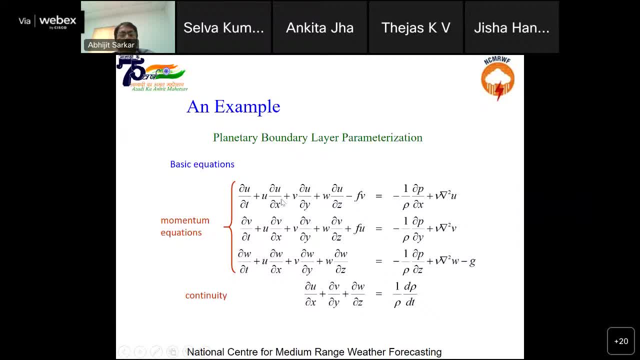 so these are the governing equations. so first, three equations are the momentum equations and then it is the continuity equation. for mass conservation equations. this? U is the total wind field, is VU, VW. they are the total wind field. now we can decompose you into two parts. one is the grid averaged party U, another is the 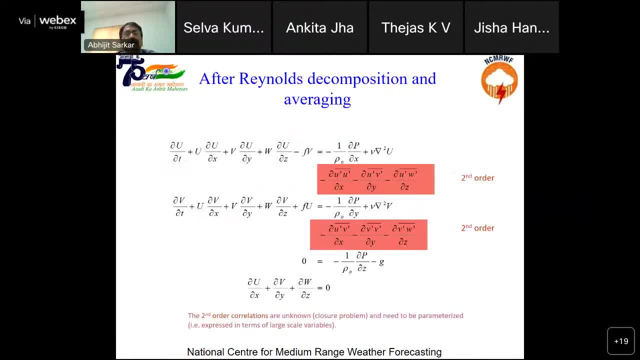 perturbation, part u, double dash, that is the sub grid scale component, and then, after Reynolds, decomposition and averaging. so these equations will be reduced to this. so this capital U, it is that grid averaged U. so this U can be resolved by the, by our model, but this U dash, V, dash. 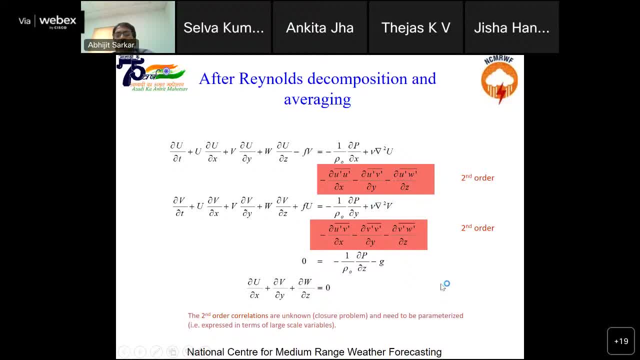 W dash. so these cannot be resolved by the model. so this highlighted part. so these part, they are very important. if we do scale analysis we will see these terms are significant and not all like U dash, double dash term. so del U dash, double dash, bar del Z. 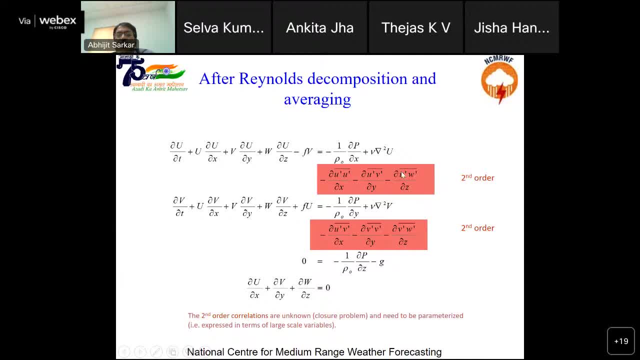 so this term is very significant. and again, del V dash W dash bar, del Z, so this term is also important, so we cannot neglect this term, so these two terms, whereas del U dash U dash bar and del U dash V dash bar, so these two, these terms, we can neglect. 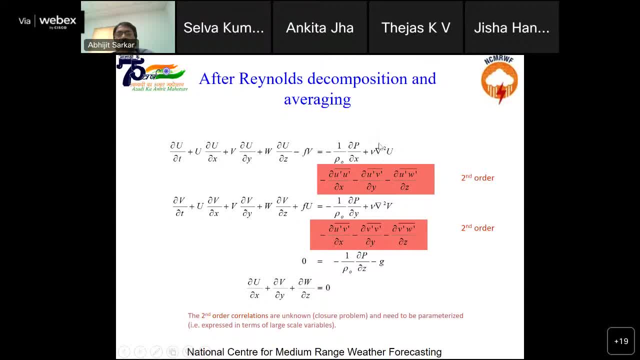 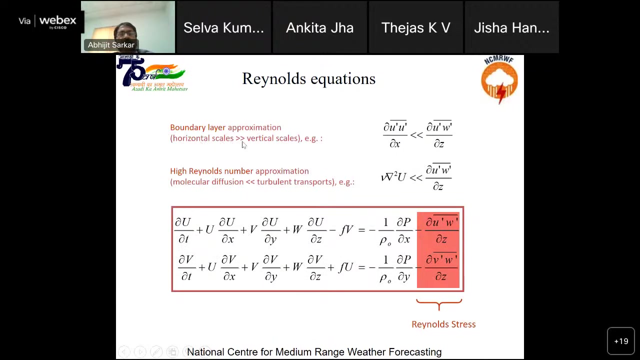 these are small terms and also the molecular diffusion terms like V del square U, so del square V, so these terms also we can neglect. so these things we can do from scale analysis. so our next thing is that boundary layer approximation in horizontals, since horizontal scales, 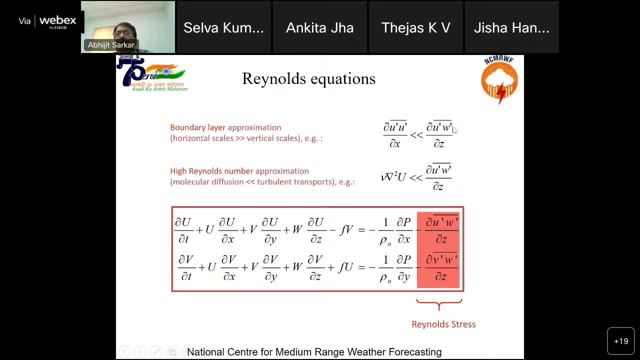 greater than vertical scales. so these vertical momentum flux, these U dash double dash term, so that we have to keep, and these U dash U dash bar term, so we can neglect. so, after making this approximation, we are getting the equation, these two equations, within the box. so now this is our final equation. 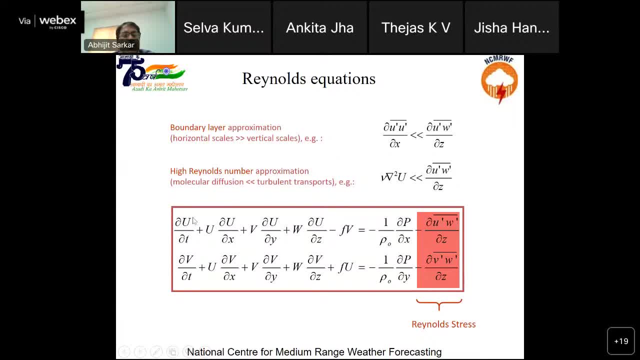 in which U is the grid average value of wind speed, V is also that grid average value of wind speed in the y direction. but how to find out these two significant terms in the last two, last two, last term? that del U dash W dash bar del z. 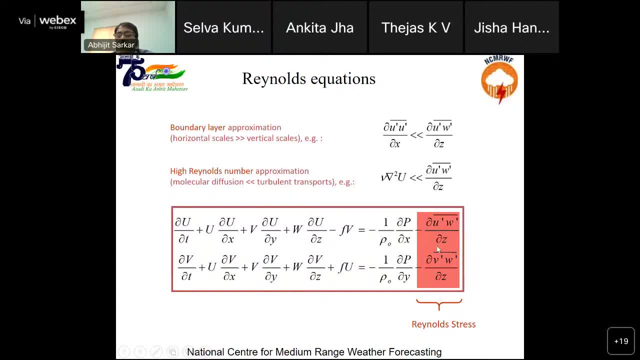 and del V dash W dash bar del z. so these two terms are important because these U dash, double dash W dash, they are V dash W dash. so they are not model variables. so they are. it is the product of two very small terms, two very small quantities. 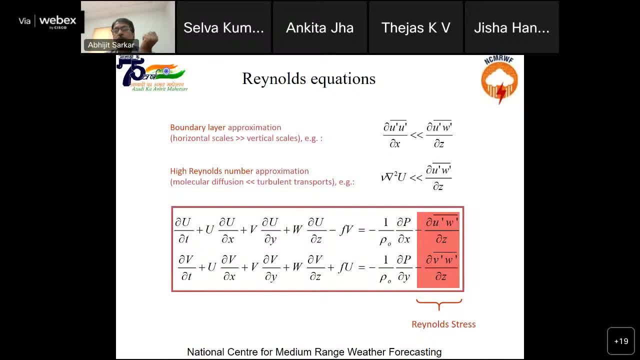 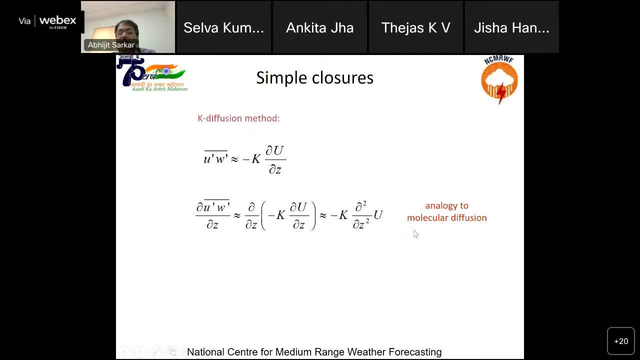 but they are giving us a significant quantity so that we have to take into consideration within the model. so how we will do that, so we will make some approximation, we will draw the analogy with the molecular diffusion. so these U dash, W dash, so they were not our model variables. 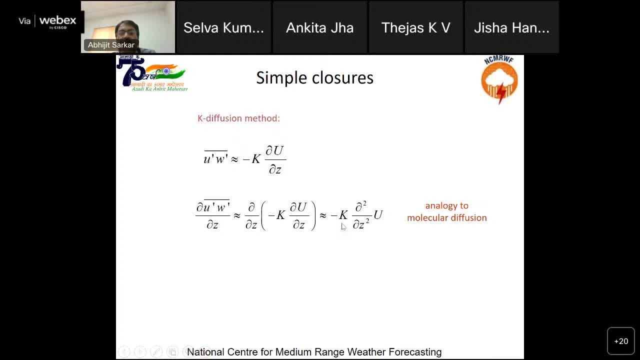 so, but this term we will write as this: U dash, W dash bar. we will write as minus K del U, del z. we will draw the analogy with the molecular diffusion. so this is an approximation, but unless we do this approximation, if we don't do this approximation, 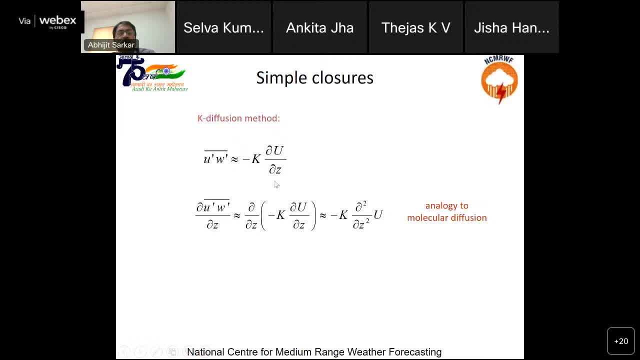 so then we will lose one term. so to account, take into account the significant effect of this small, small scale phenomenon, we have to make some approximation, and here we call it is the closure. we are solving the closure problem. we are now, when this is expressed in terms of model variable, 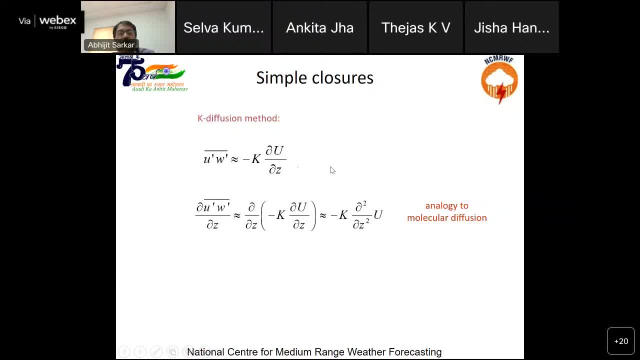 so there are. now my equations are closed. so now the number of equations and number of unknowns are becoming equal. so now we can solve these equations. so we are solving this closure problem. so this is called parameterization, so that collective effect of this small scale, sub grid scale phenomena. 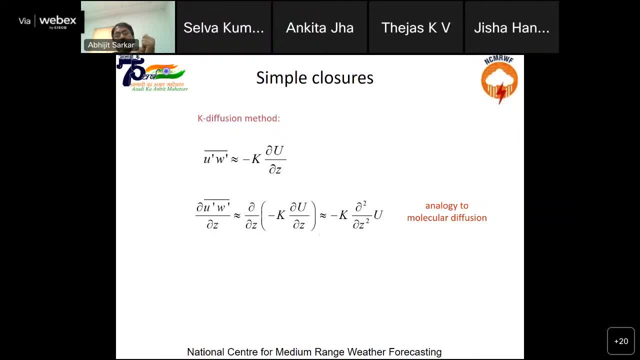 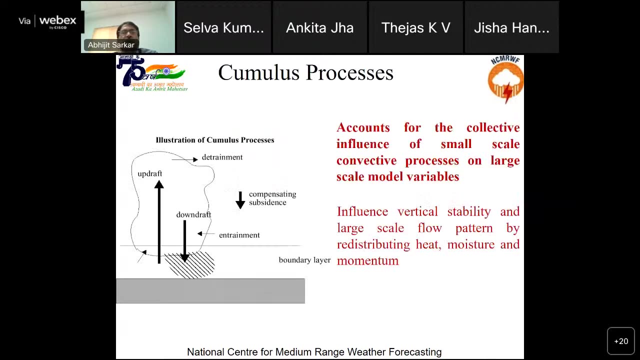 we are expressing in terms of large scale variables. so this method is called that parameterization of physical processes. next comes cumulus process. it accounts for the collective influence, for the collective influence, for the collective influence of small scale convective processes on large scale model variables. the objective of this cumulus processes is 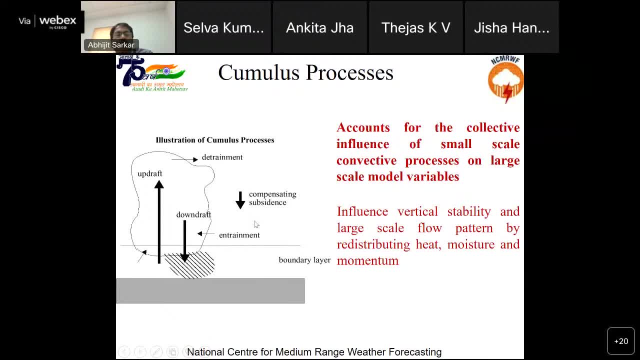 to reduce the instability in the atmosphere, but its byproduct is rain. so if we parameterize this cumulus process, so then it will give us this convective rain. also. it influences vertical stability and large scale flow pattern by redistributing heat, moisture and momentum. then cloud microphysics. 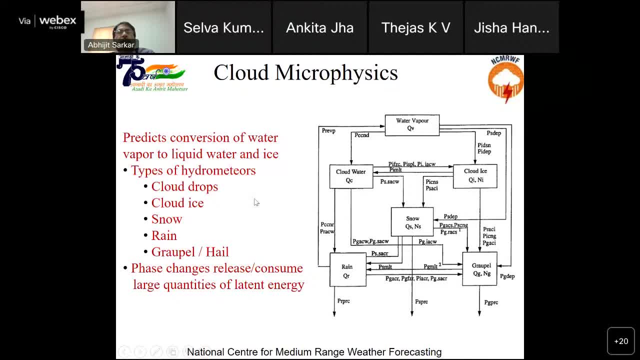 so the mechanism through which the different types of hydrometeors are formed. so that is this cloud microphysical process, so different types of my hydrometeors we can take into account, like cloud drops, cloud ice, snow, rain, grow, pale hail. so so many physical processes we have to parameterize. 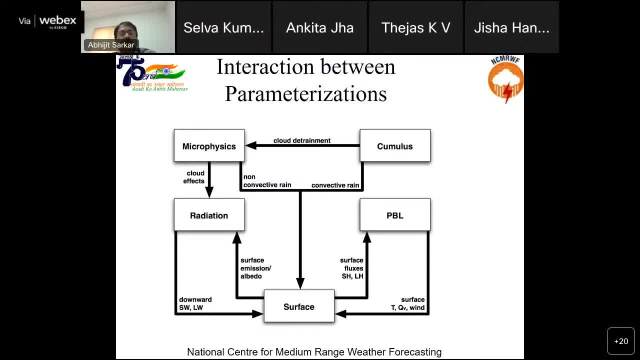 and then then then all these processes are interrelated with each other. if our parameterization of cumulus convection is not good, so then the cloud cover prediction also will not be good. and it cloud cover prediction is not good, so then rain. rain prediction will be will not be good. 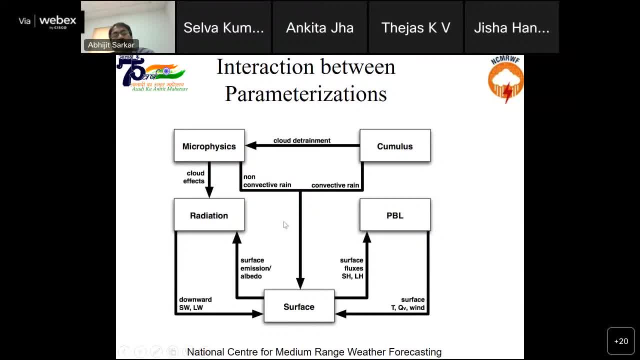 and then incoming short range forecast will be bad. and if incoming short range forecast, short range radiation forecast, is bad, so then temperature forecast will go bad. and then again, if temperature forecast goes bad, so then how much will be evaporated? how much water will be evaporated? so that will also that forecast also will go bad. so all these 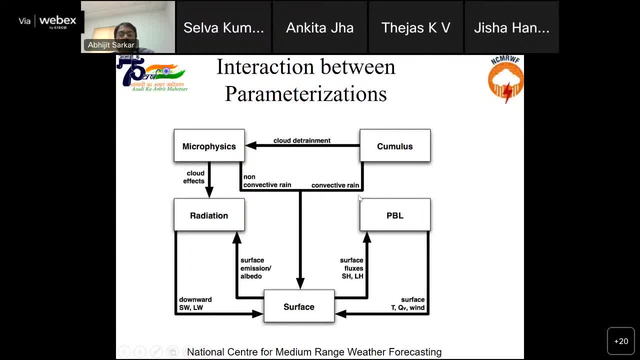 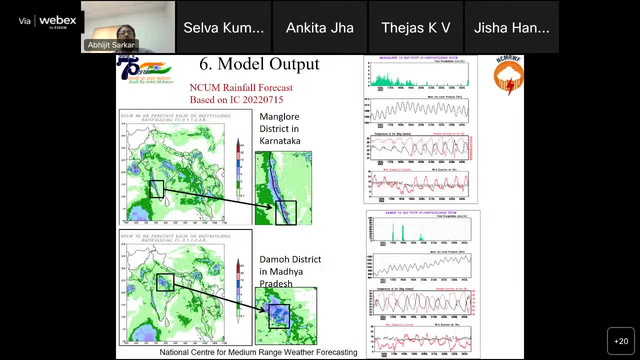 physical processes. they are interrelated with each other, but here a lot of approximations and assumptions are associated and therefore lot of errors and uncertainties also will be there. so we can see. finally we will get that model output, and model output are presented in this format, in the form of weather map or location specific format. 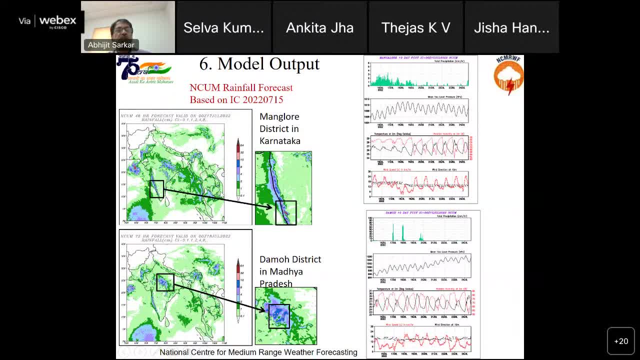 in the form of meteogram. so this is today's model forecast, our global model forecast over western core. i am highlighting the region over the western coast. we can see the region of mangalore and that neighboring region is predicted to get a very heavy rainfall. our right side location: specific forecast. 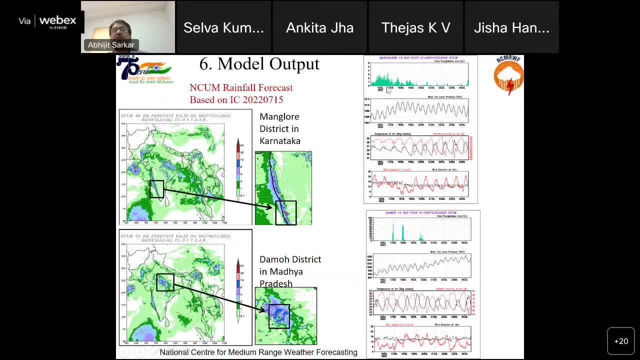 by meteogram is also showing that that on 16th and 17th it will get a very heavy rainfall. and again over the central india we can see thataly damo district, that region is getting very heavy rainfall and same thing is reflected in our rewrites. 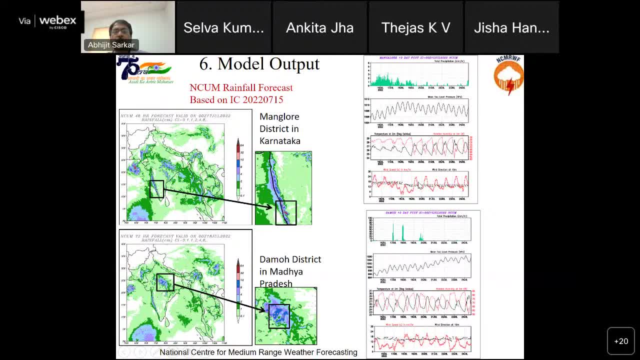 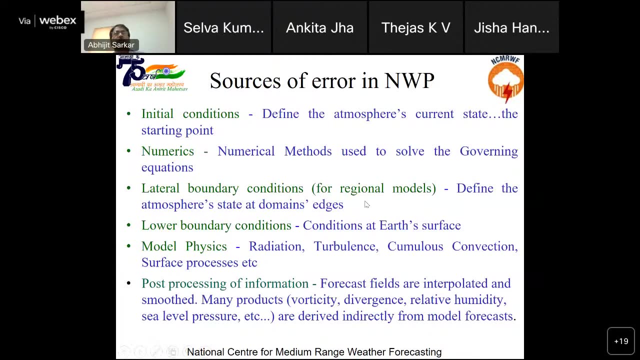 meteogram also, but these plots do not tell us that how much uncertainty or associated, how much uncertainty or error associated with 2024 year is migrating from lingam and change to april and is with these forecasts. So we can see that sources of error in NWP include initial conditions. 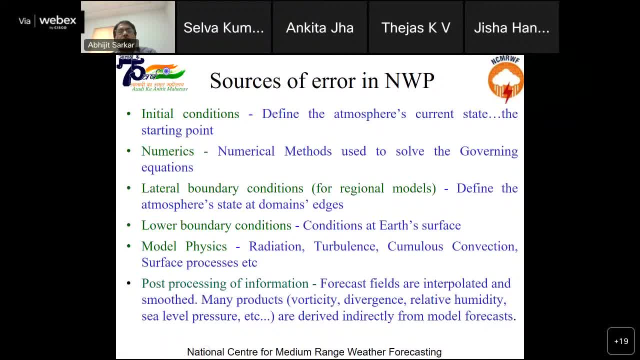 starting from initial conditions, Each step of NWP is having error or uncertainty. Then numerical methods used to solve the governing equations. Then error in specifying the lateral boundary condition and lower boundary condition, In parameterizing the physical processes And even the post-processing of information, also because we have to do interpolation. 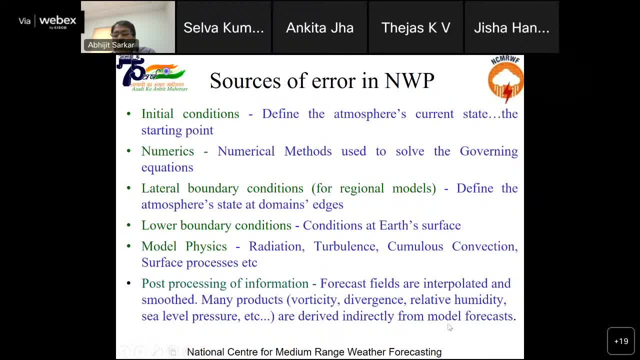 And then many products are derived indirectly from model forecasts. So at each step of the method of numerical weather prediction there is error or uncertainty And we need to inform this uncertainty or error associated with model forecast to the users or to the forecasters. 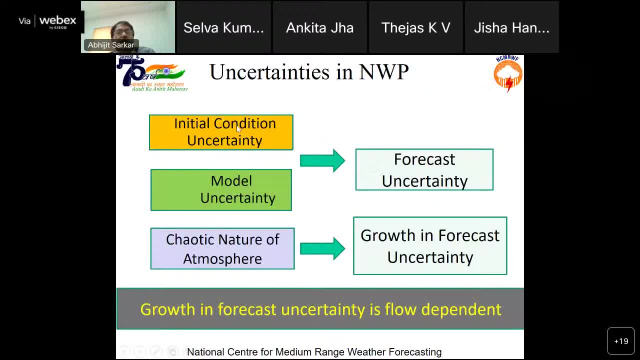 So we can see that there is uncertainty in the initial condition And there is uncertainty in the model formulation which gives forecast uncertainty. And since atmosphere is chaotic in nature, that uncertainty grows with time, So there is growth in forecast uncertainty. 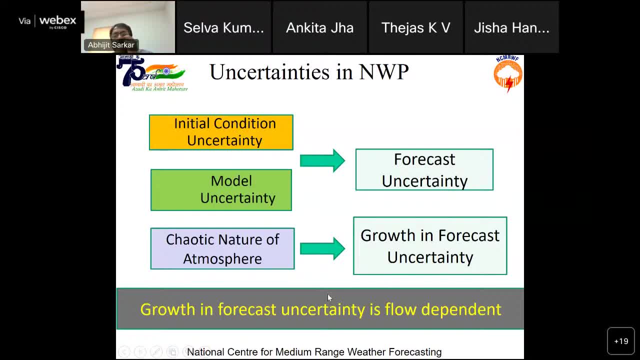 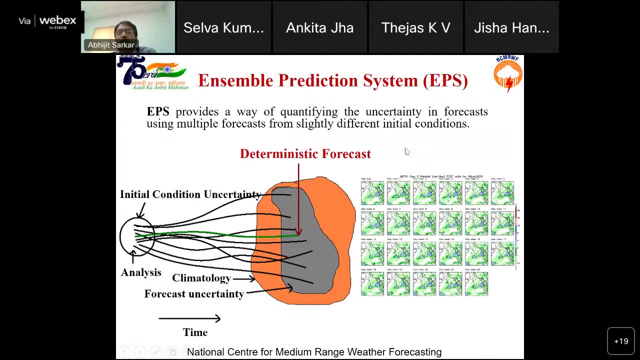 And how fast that error will grow That is not fixed. That again will depend on the atmospheric condition. Or we can tell that growth Growth in forecast uncertainty is flow-dependent. So along with the forecast we have to quantify the forecast uncertainty also. 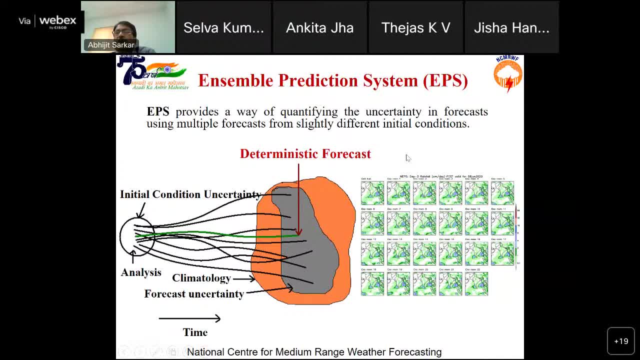 And that forecast uncertainty we have to communicate to the users or forecasters. That will help them to make better decision-making, to take better decisions. And then ensemble prediction system. it provides a way of quantifying the uncertainty in forecast by using multiple forecasts from slightly different initial. 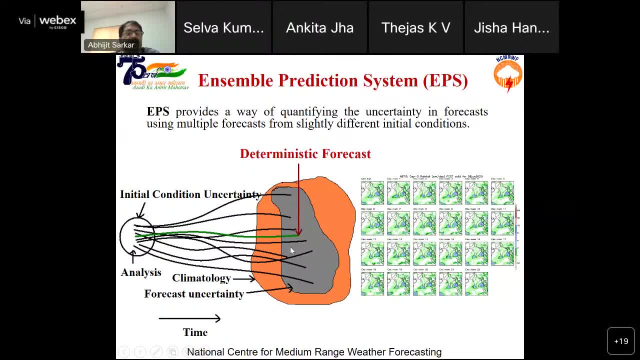 conditions In ensemble forecasting system. that whole uncertainty in the initial condition is covered by these multiple initial conditions And then from these multiple initial conditions they are slightly different from each other. From these slightly different initial conditions, multiple models run. Actually, these all are same model. 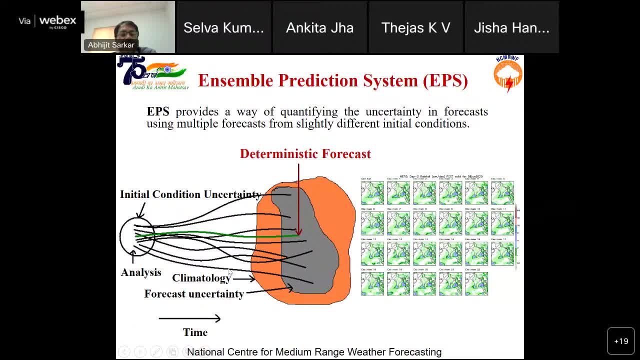 They are very similar but they are not identical. All the models are little bit patterned So it is very difficult to take into account the model uncertainty. So this initial condition, it covers the whole uncertainty range And from there we are getting multiple forecasts. 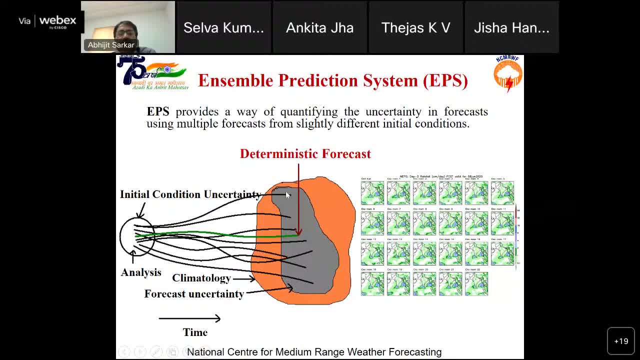 So we are getting a forecast uncertainty. Our NCMWF Global Ensemble Prediction System has 23 ensemble members, So you can see. so there are 23 forecasts And all the forecasts are very similar to each other, but they are not identical. 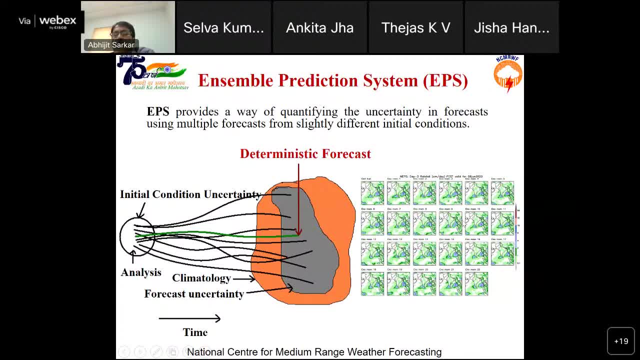 And from these forecasts, from these multiple forecasts, we can issue probabilistic forecasts So we can communicate that uncertainty in the forecast. in terms of probability, If there are 20 ensemble members and five ensemble members predicts rain, then you can tell there is 25% probability of rain. 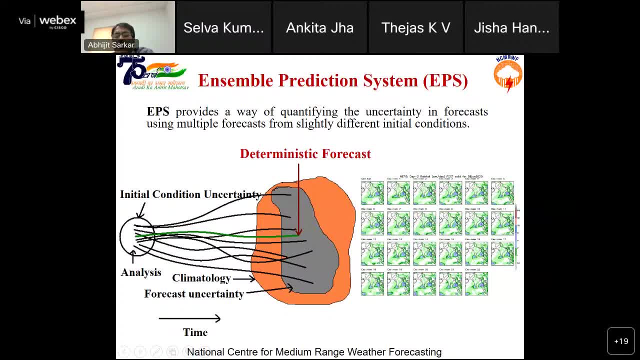 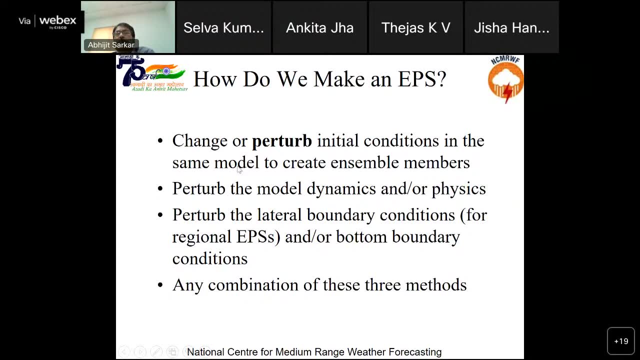 So this way we can communicate the uncertainty in the forecast in terms of probability. How do we make an EPS So that already we have seen, We can change or perturb initial condition. We can perturb the model dynamics or physics, We can perturb the lateral boundary conditions. 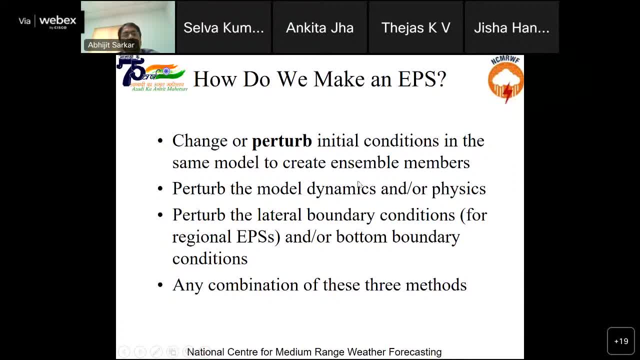 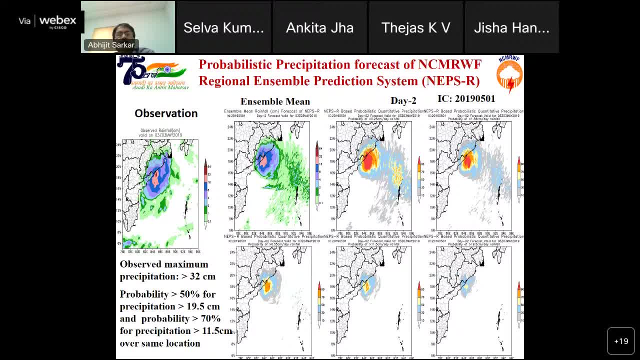 Or after running this ensemble prediction system So we can express the model forecast in this form. In the left side you can see that observation. So it is the precipitation at the time of Foney tropical cyclone. On the right side, first slide, is ensemble mean day two forecast. 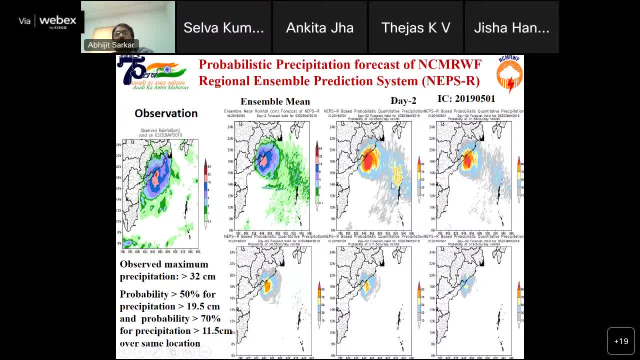 And next one is probabilistic forecast. So this forecast we can interpret in this way: that over this Orissa-Andhra Pradesh coast the probability of rainfall greater than 0.25 centimeter per day is greater than 90 percent. So this way we can interpret or this way we can communicate. 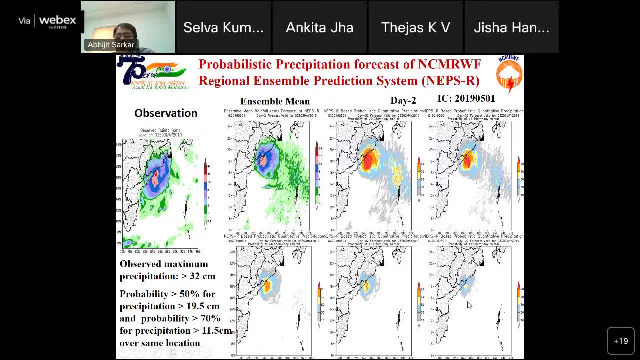 that uncertainty in the forecast For the last panel, if you see. so we can tell that probability of rainfall greater than 19.5 centimeter per day, which is considered to be extremely heavy rainfall. So this is between 50 to 70 percent, or greater than 50 percent. 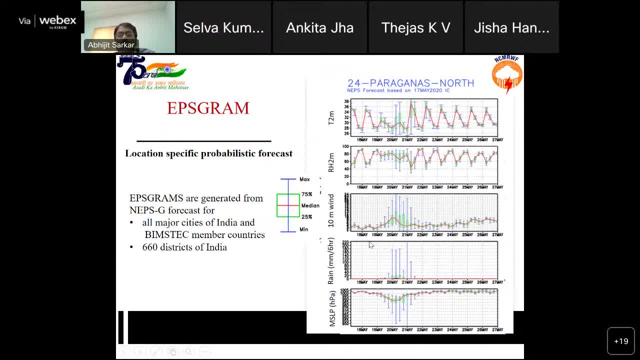 So then, location specific forecast, which I showed previously, in the form of meteogram. So, in case of ensemble prediction system, we can express this location specific forecast in form of EPS graph, So here, with the help of a box whisker diagram, so the top of this vertical line. 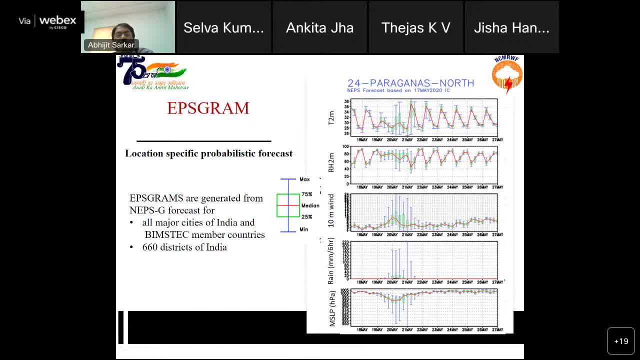 it is giving the maximum amount that any ensemble member could predict and bottom horizontal line is blue line. it is giving the minimum amount that any ensemble member can could predict and the red one is giving the median. So we can see from this forecast that fourth panel from the top. so it is giving us the rain forecast in six hours. 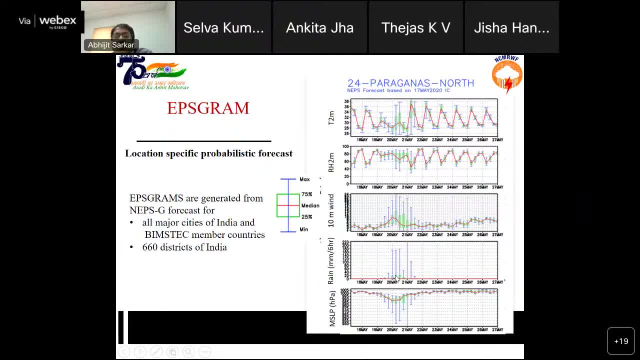 So we can see that the roof of the green box on 20th May. So it is touching this 20 millimeter, this horizontal line. So we can tell that 75 percent members have predicted the rainfall below 20 millimeter in six hour. 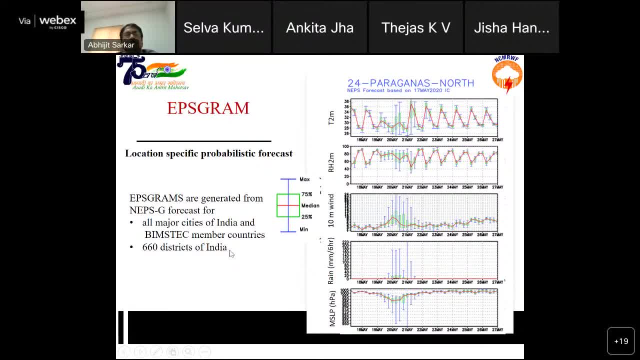 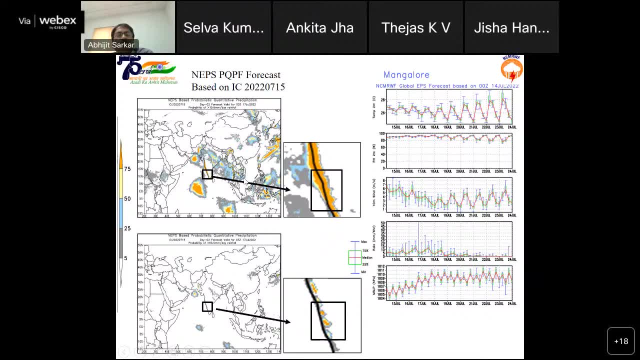 this way we can interpret- and this from the today's initial condition that heavy rainfall, which i showed this deterministic forecast in the form of probabilistic forecast. we can show in this way: so left side it is the probabilistic forecast and right side it is the location specific probabilistic forecast. 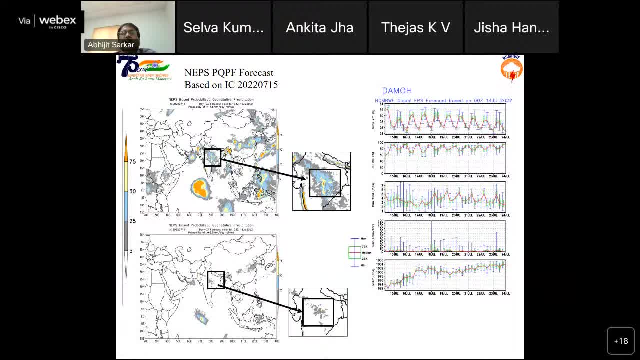 over mangalore, similarly for the damo district. so this is the probabilistic forecast. left side it is the special distribution of rain, probabilistic forecast of special distribution of rain, and right side, again it is the in the form of ups gram, the probabilistic forecast of. 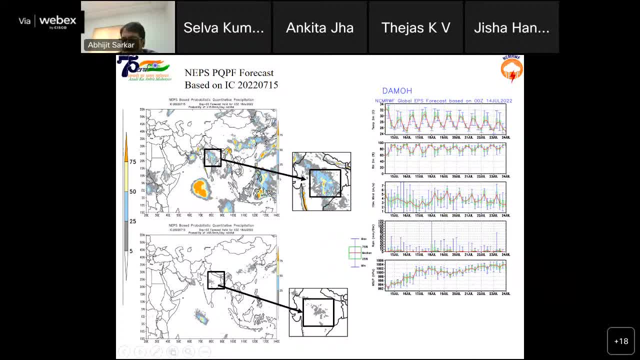 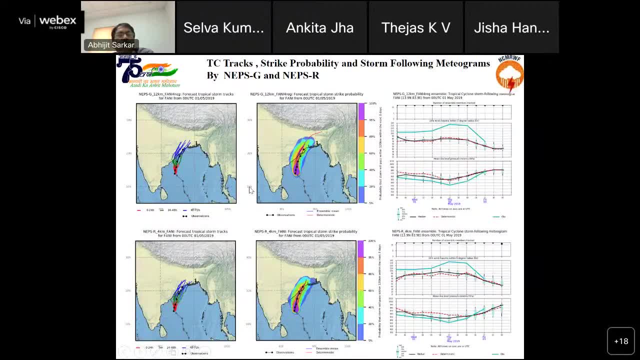 rate probabilistic forecast at a particular location. similarly, the cyclone forecast also in in place of one track in the in ensemble prediction system, we will get many tracks so that the disaster managers so they will know that what is the probability of landfall at different places. so this middle panel, it is giving the strike probability of.